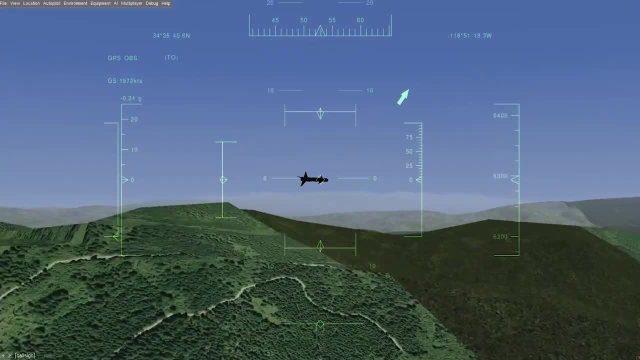 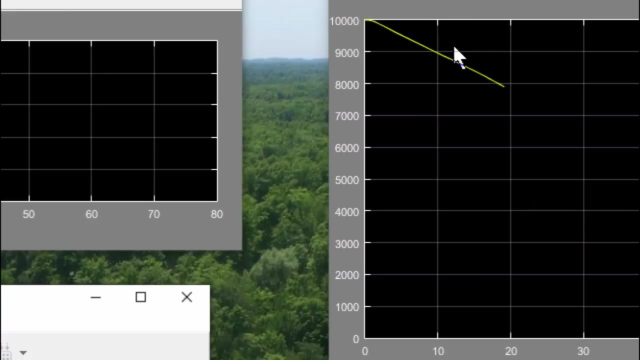 how you can work with navigation, like latitudes and longitudes, for example, and how to calculate the guidance commands based on results from the navigation Kalman filter. So I will teach you a lot of aerospace topics and you will learn quite a lot in this video. This. 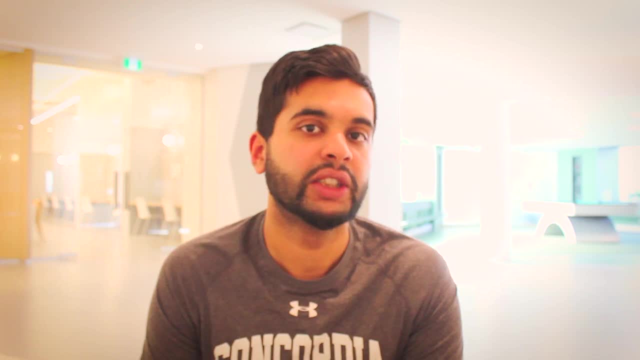 is my special video for 2020.. This took me a long time to complete So, with that being said, I hope you guys enjoy it. Let's begin. So let's say: it's a Saturday morning and you want to go. 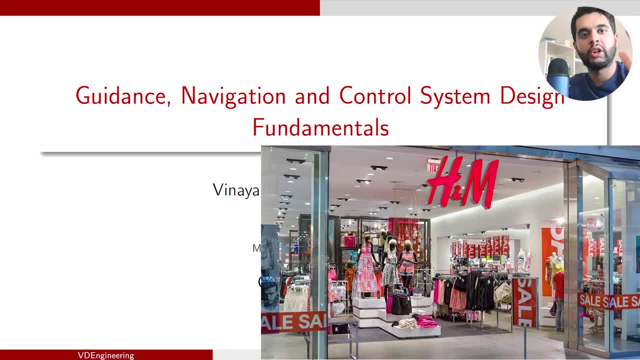 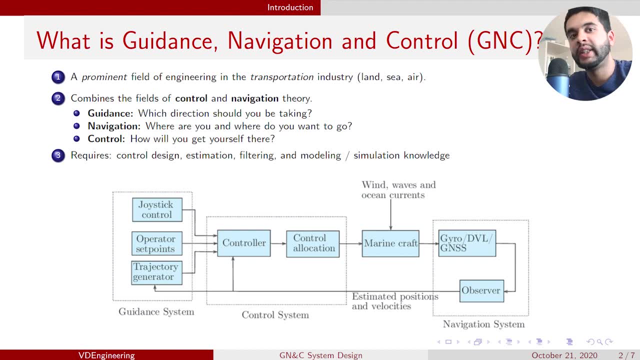 shopping at H&M to buy a jacket. Let's say you have to go north. That would be the guidance command. The shop is located 10 miles away from you. The shop is located 10 miles away from you And you have to use the GPS on the car to take you there. This would be the navigation commands. 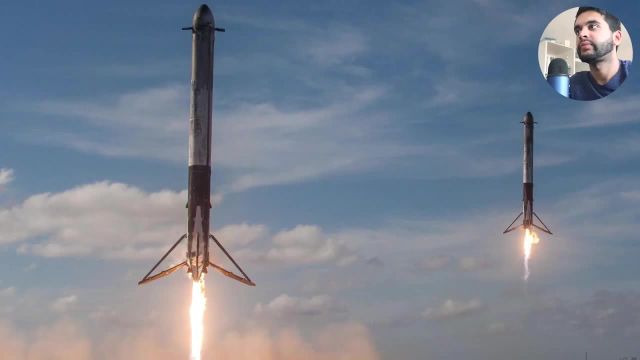 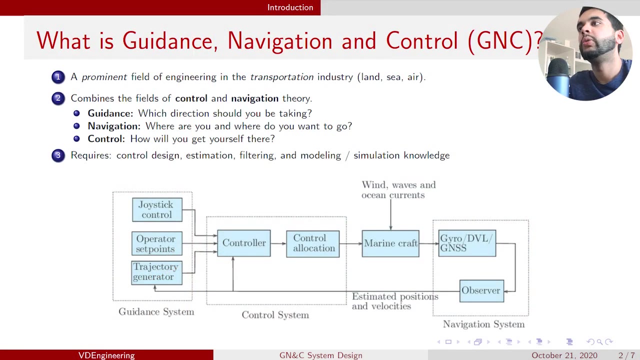 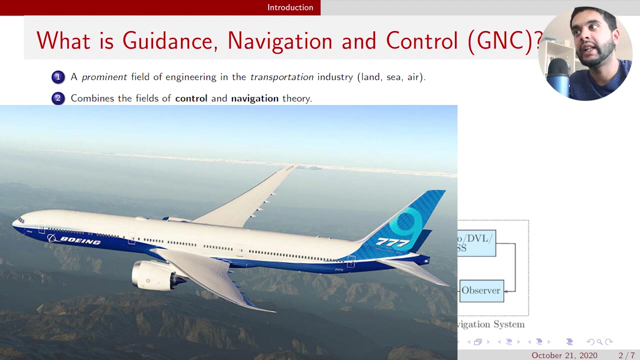 So the GPS will tell you to turn left or to turn right. Lastly, how will you get yourself there? Will you walk? Will you take the bus? Will you drive? That's your control command. So GNC is a very interesting aerospace field and it's used every single time a new airplane is designed. 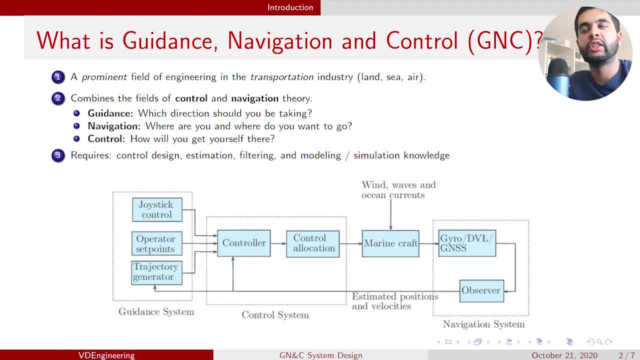 You need to have knowledge of control system design, estimation, filtering, along with modeling and simulation, And in this video, I'll be teaching you all of that in detail. If you look at this picture here, this is taken from the NASA Engineering Safety Center, or NESC. This is the standard GNC. 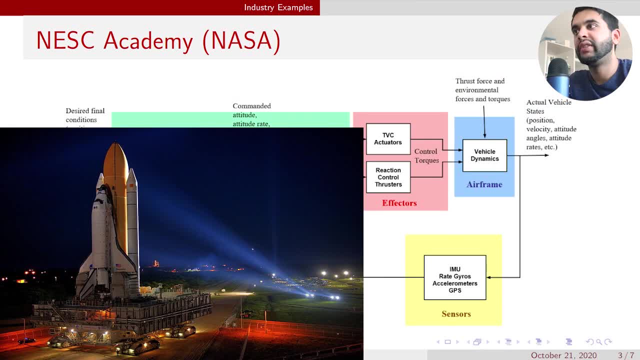 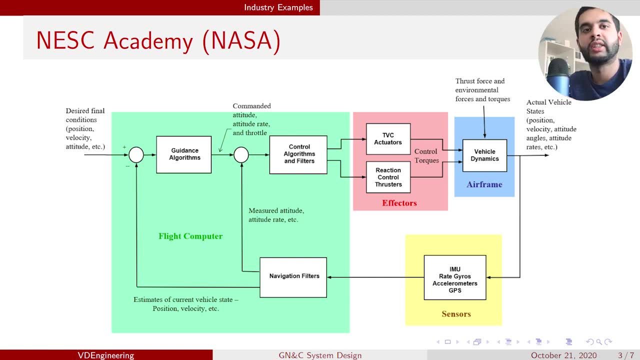 algorithm for a launch vehicle or a rocket, for example. You have the flight computer, which calculates the guidance commands and tells the controllers what to do. You have the effectors, which are the vehicle actuators. Then you have the vehicle airframe, which is the 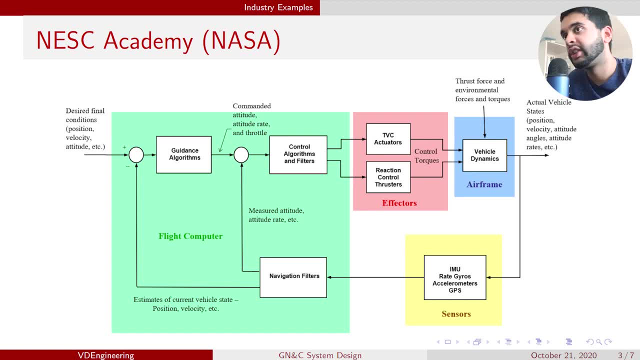 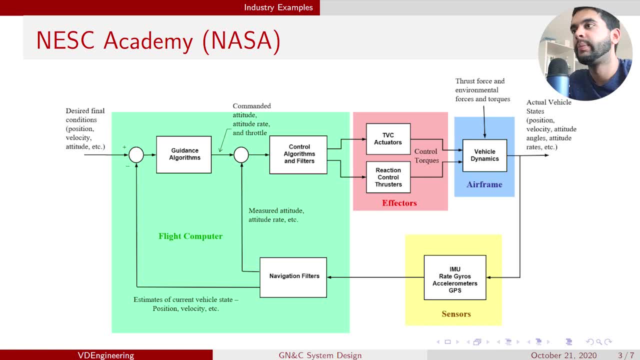 or a GPS. So the rocket is connected to sensors, for example an IMU or an IMU. This then sends commands back to the Kalman filter, Then the navigation system tells the guidance systems what to do and the whole thing works at the same time. So this is a GNC loop, in different words. 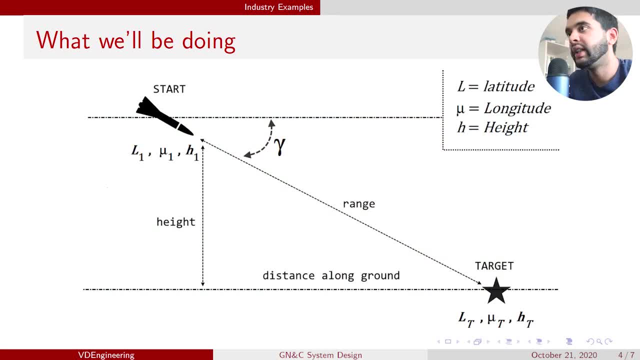 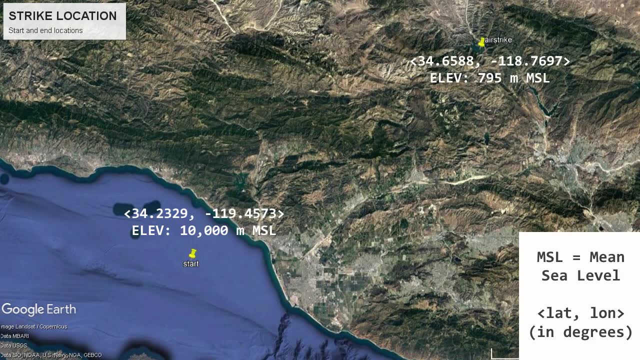 So for this video, what we'll be doing is that we'll be doing a missile strike. The missile starts somewhere in the air and it has to come all the way down to hit a target on the ground. The target will be set by us. We'll be setting the initial latitude, longitude and the height, along with 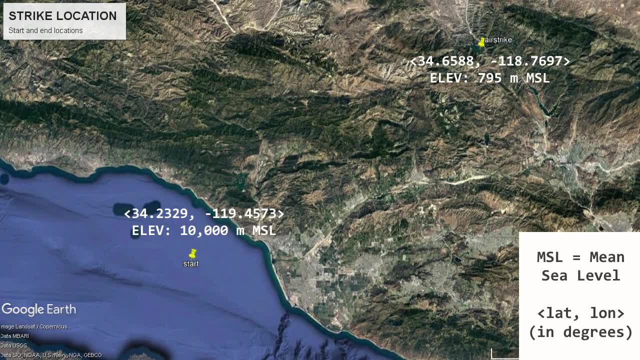 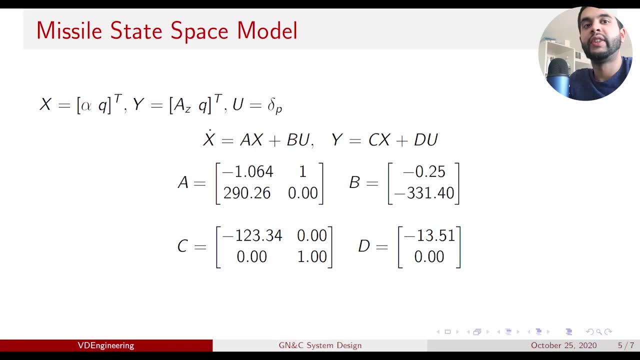 the target latitude, longitude and the height, And we'll be using the whole GNC design procedure to calculate the flight path angle which you need, which is this gamma, as you can see there, And it's very interesting. So here we have the missile model. This is taken from a company. 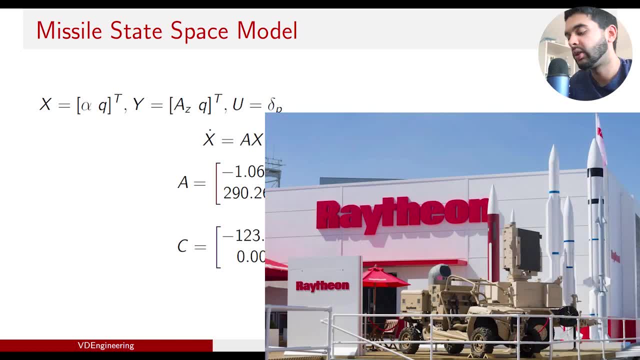 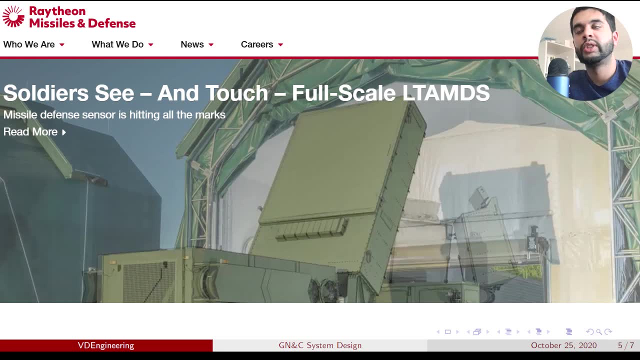 called Raytheon Missiles and Defense. They are based in Tucson, Arizona, along with many other locations around the US. It's a large American defense contractor. They have built all the missiles which are made in the United States. They have built all the missiles which are 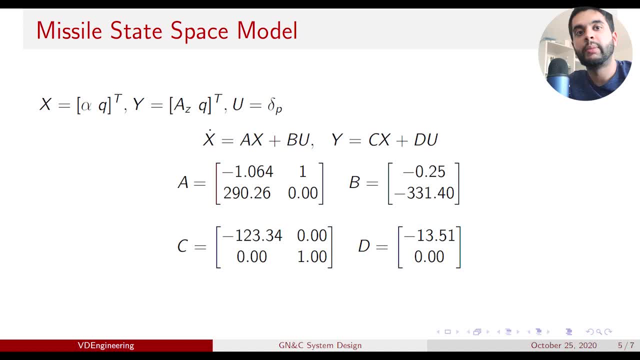 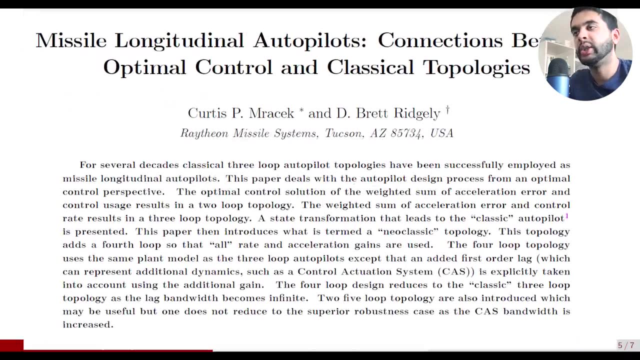 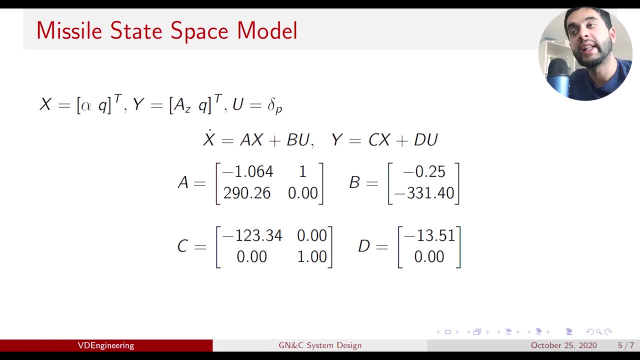 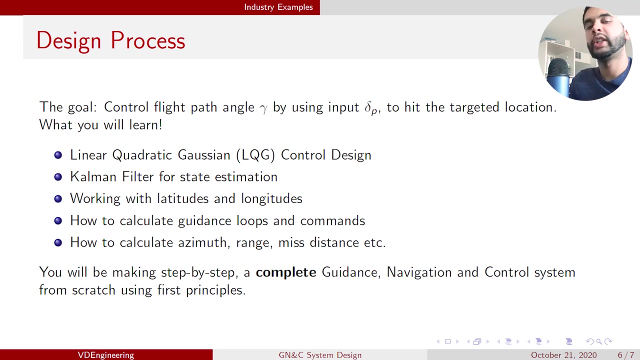 made in the United States. It's a very big company. It's a very amazing company. This is taken from a paper which was published by Raytheon Missiles and Defense, by two scientists, and that'll be linked in the description below. So in this video, you will learn how to control the flight path angle gamma by using the missile actuator. You only have one input there to hit the targeted location. So what you will learn? you will learn LQG control design, You will learn column and filtering, how to calculate latitude and you will learn how to calculate the latitude. So let's get started. 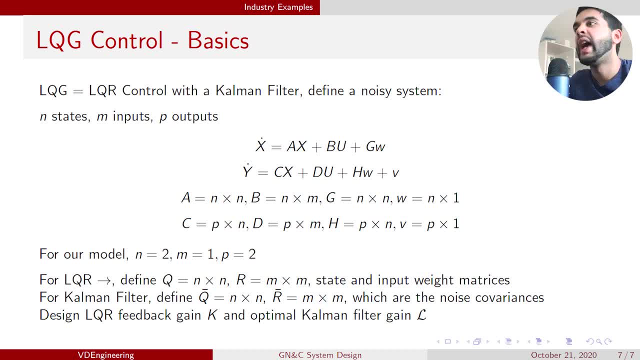 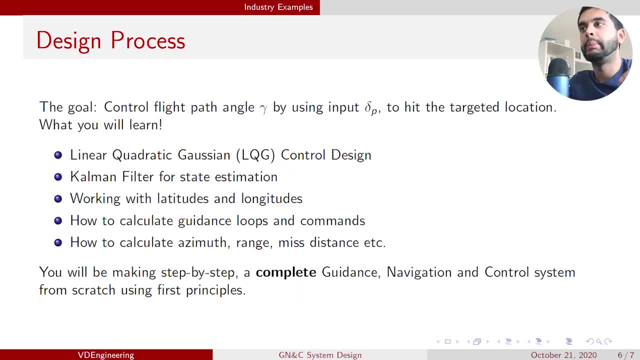 And lastly, how to calculate standard things in aerospace GNC, For example, azimuth, range, distance, blast zone, accuracy and so on. So you'll be making step-by-step, a complete guidance, navigation and control system from scratch. Let's start. 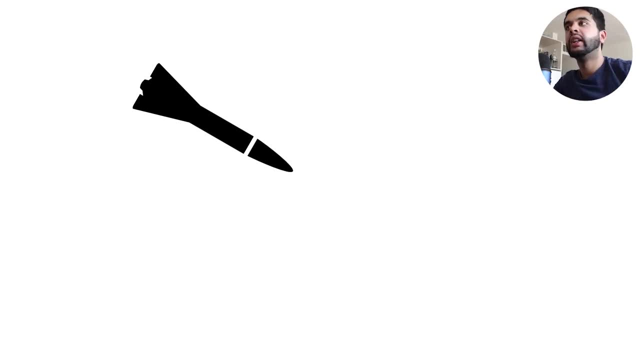 Just want to introduce you to missile defense and some of the notation and terminology used in missile engineering and also aerospace in general. So this is the horizon. we have the body frame, XB pointing forward and ZB pointing down. this is only a 2D, so we will not look at why, for example here. 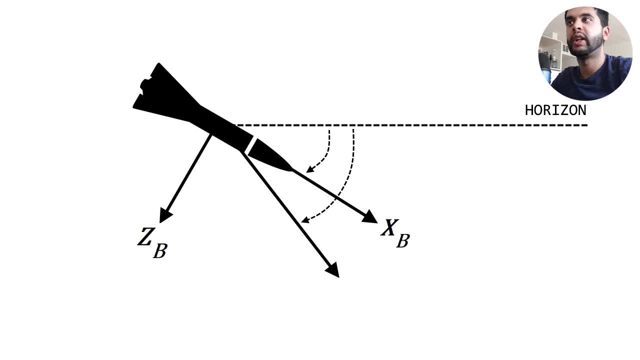 you have two angles: the pitch angle from the horizon, then you have gamma, the flight path angle, and then you have alpha, the angle of attack, which is in respect to the body frame and the velocity. so the missile is actually moving this way. for example, you have these angles which you should know: The flight path angle. 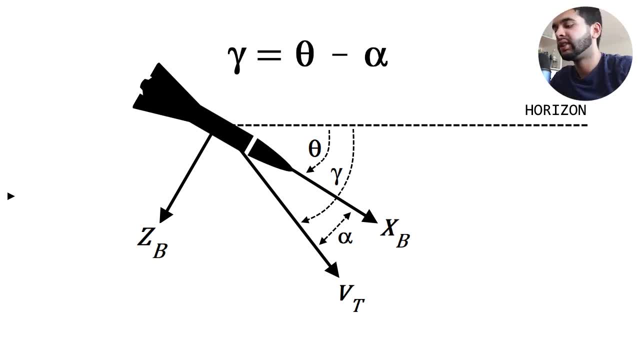 is equal to the pitch angle minus the angle of attack. and this is this is a rule. it has to be done this way, and when you design your GNC algorithm or any aerospace control system, you have to use this notation here. So we have the start. 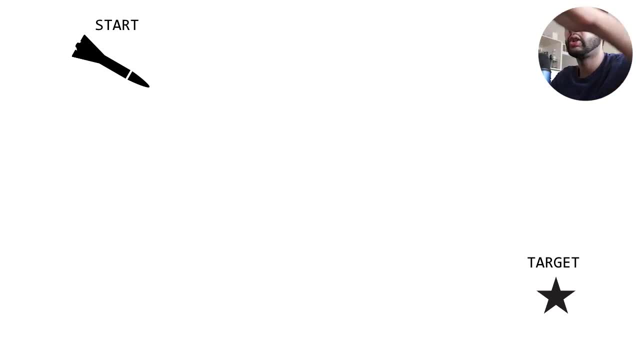 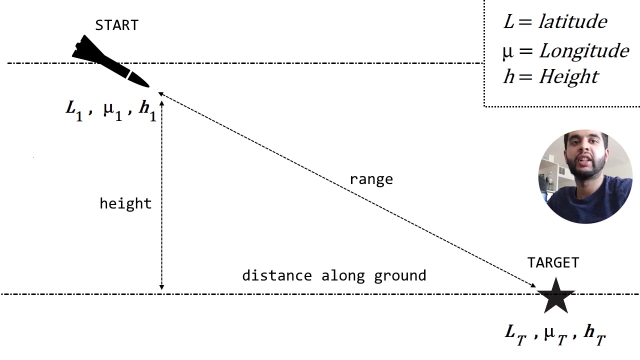 at a target. you have the start point at some location, you have the target at some location. there you have latitude, longitude and height, which you have to define yourself. you have so along the floor, you have the distance there and you have the height right. so, with with the Pythagoras theorem, 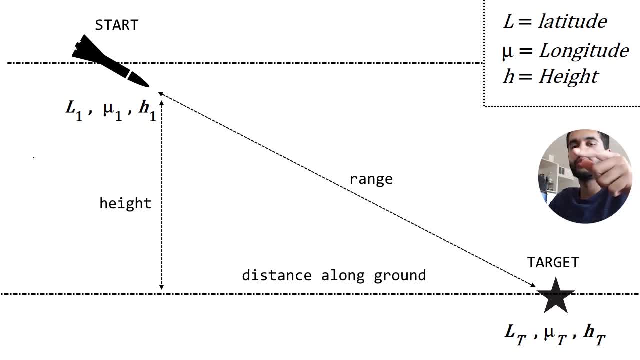 so, for example, you know, X squared plus Y squared equals Z squared and the square root of the whole thing. after some time you will have a midpoint here. so, for example, it will be a different latitude, longitude and height because obviously the missile is moving from the air. now. this problem is not very straightforward. 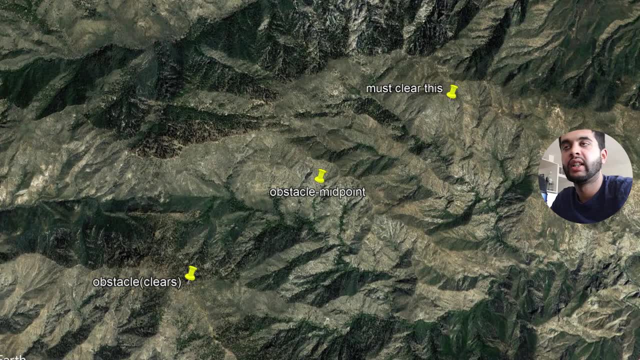 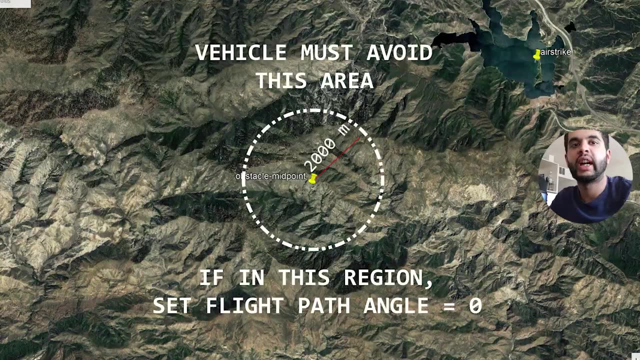 I made it a bit more challenging. you have to clear an obstacle in the way. so, because this is in the real life, right, like obviously if you design a missile, you can just like make it go straight the entire time because it might hit something else. so you have to evade obstacles in the field of aerospace. this is called. 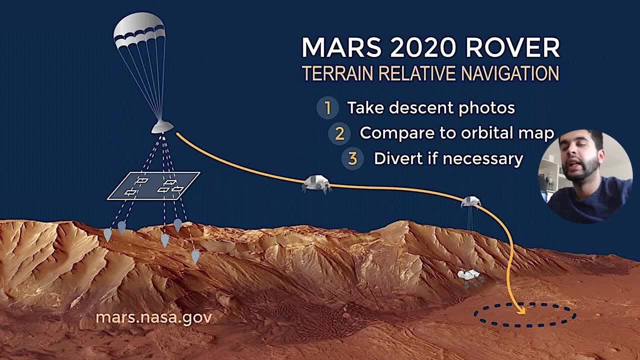 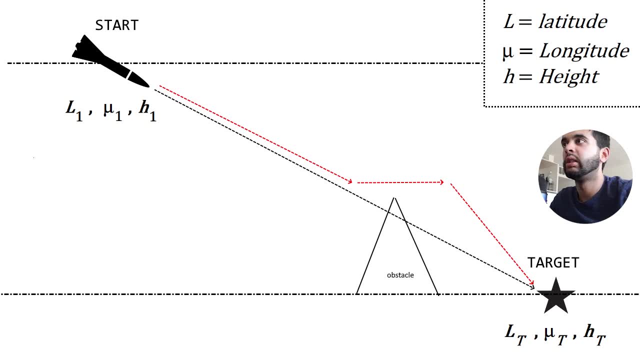 brain, relative navigation, TRN. so this looks at obstacles on the ground and how to escape them. so we'll be firing the missile from here and it will be coming, coming, coming, and then it will pitch up, it will evade the obstacle and then hit the target. 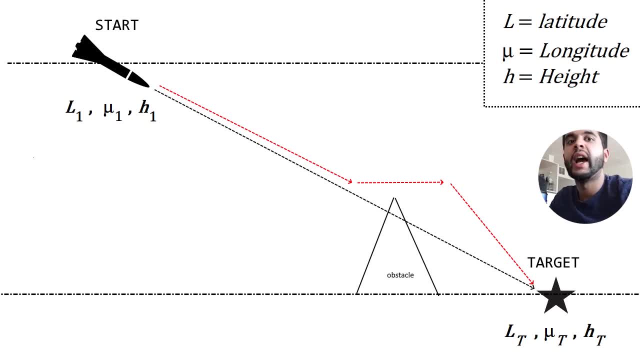 So the obstacle location will be defined by us and you will use the GNC loop to calculate how to evade the target, so it'll not be done like a brute force method. we'll be using a very smart algorithm to do this and it'll be very interesting. so let's begin. 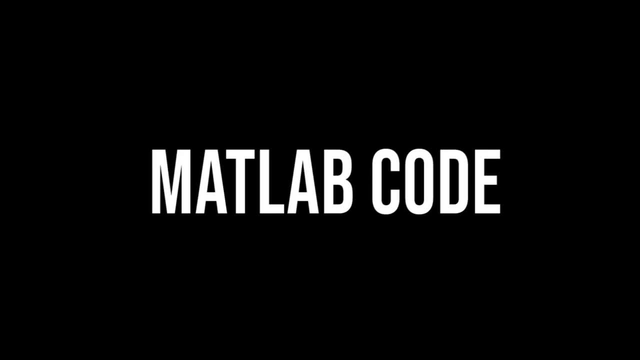 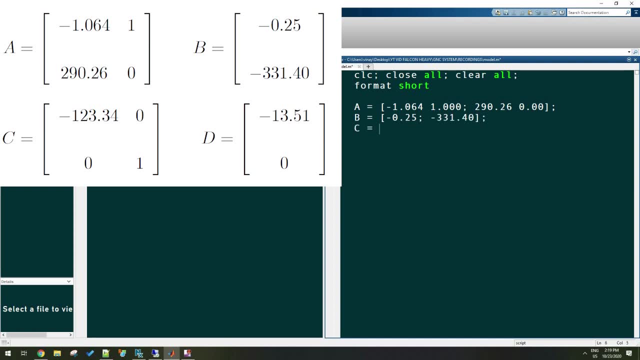 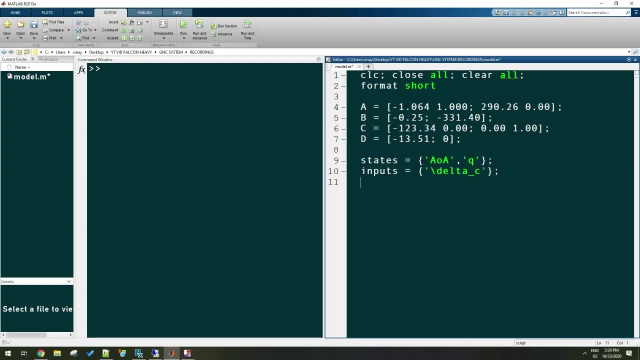 let's define the MATLAB code. so first you can define the system matrices a, b, c and d, which you can see there and it's taken from the paper itself. then you can define the states, what they are, the inputs along with the outputs, then the state space model by ss command. 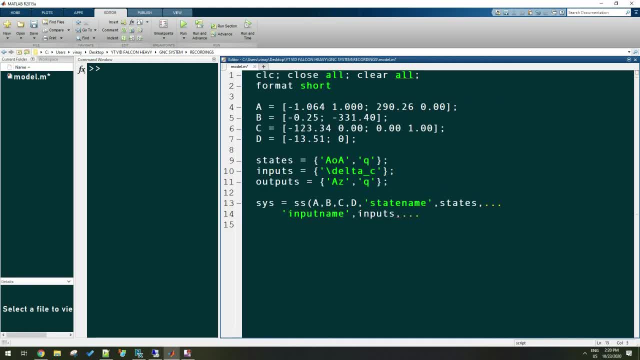 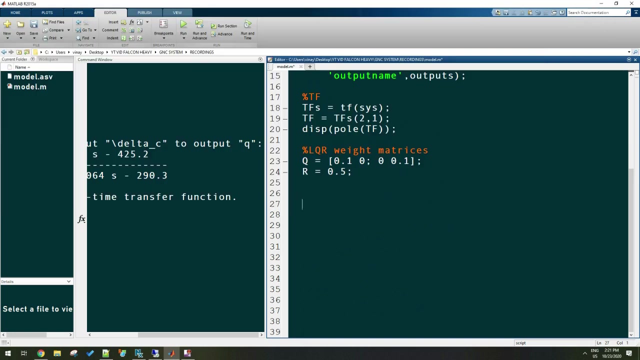 define the transfer function and plot the poles to see if it's stable or not, set the LQR matrices q and r and then run what you have so you can see the transfer function there. next, you can calculate the LQR feedback by using the LQR. 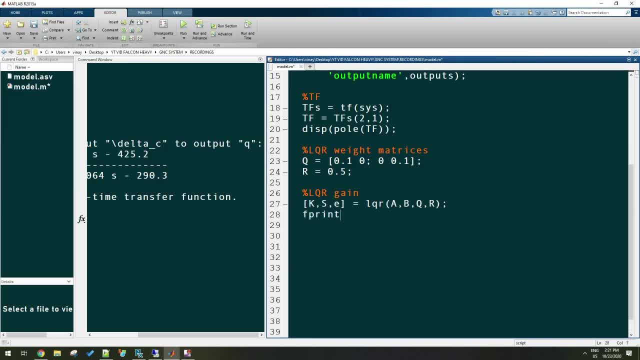 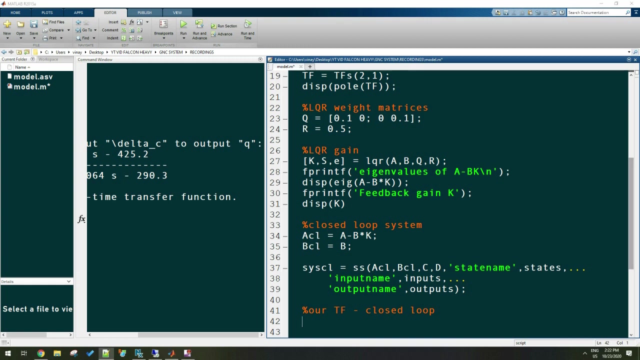 MATLAB command and then print the eigenvalues of a minus b, k, so that your closed-loop system- so you can print the gain as well- then you calculate the closed-loop system there and define it once again by using the SS command. when that's done, you can calculate the closed-loop transfer function, so it'll. 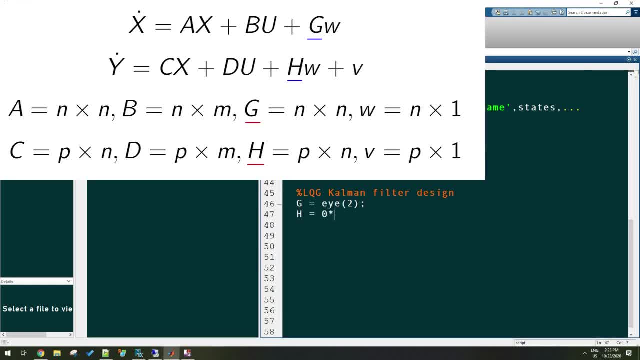 just be a minus b k, right, so you can use the same command there. next we can calculate the Kalman filter. so for example, we have to define first G and H. G is the identity matrix and H is the zeros. define the noise covariance is Q and R, which I've done before in my MIMO Kalman filtering video. then define: 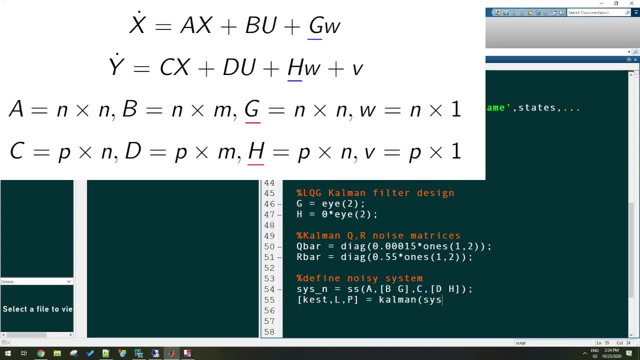 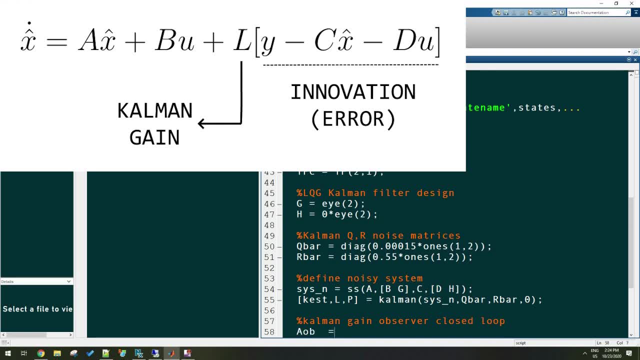 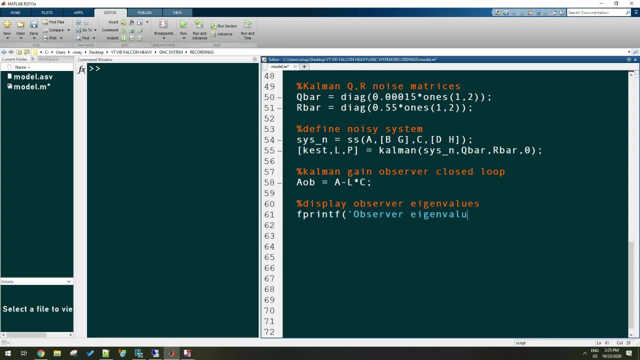 the noisy system and then use the Kalman command to calculate the L matrix, which is the Kalman gain. this is once again a steady-state Kalman filter, because it's very fast. then you can find the observer poles by doing a minus L times C, and you can print them as well very easily. so they 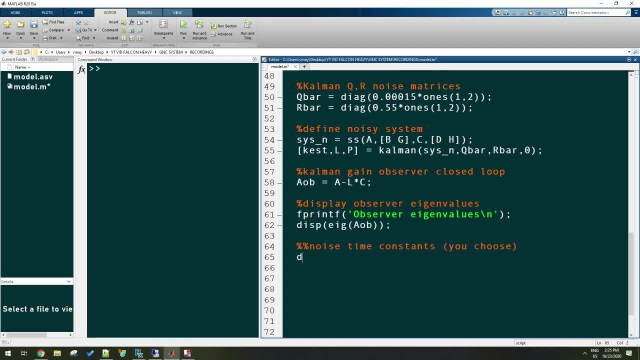 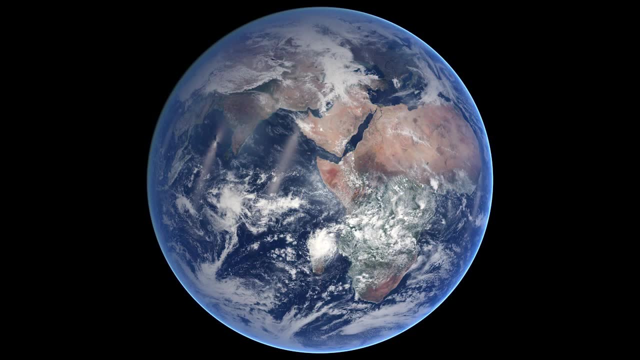 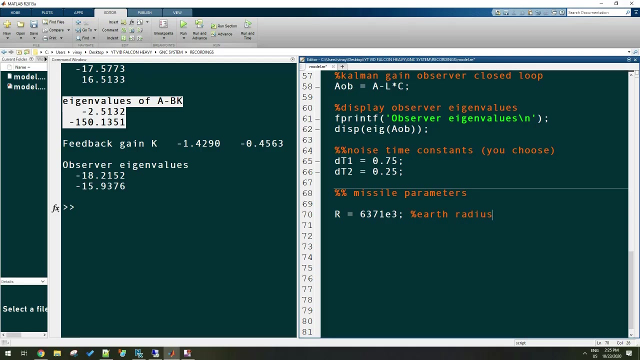 should be stable and very quick. next, you can define the noise time constants which we'll use after in Simulink. so just define it there. and lastly, you can now define the missile parameters. so you have first all the control results. you can define the velocity and the velocity radius there. this value is approximate. 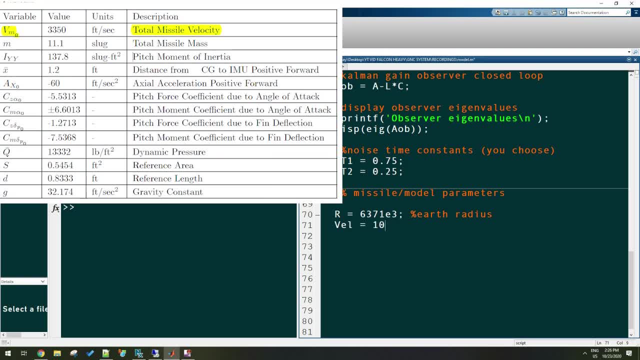 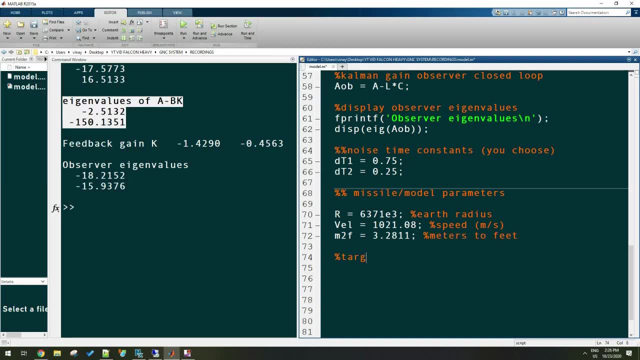 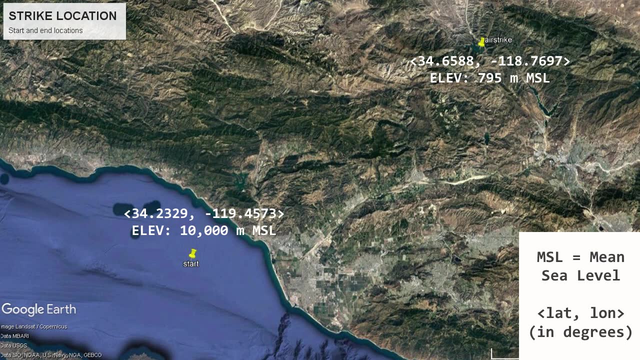 because we all know the earth is an ellipse, it's not a perfect sphere. the missile velocity is taken from the paper and it's constant at about one kilometer per second. the target location can be set in degrees latitude, longitude and height. the initial location, the same procedure, degrees latitude, longitude and. 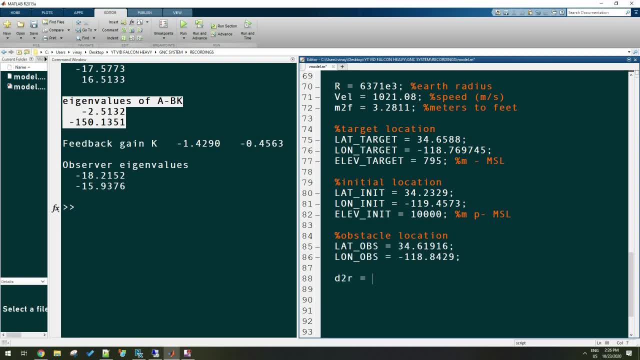 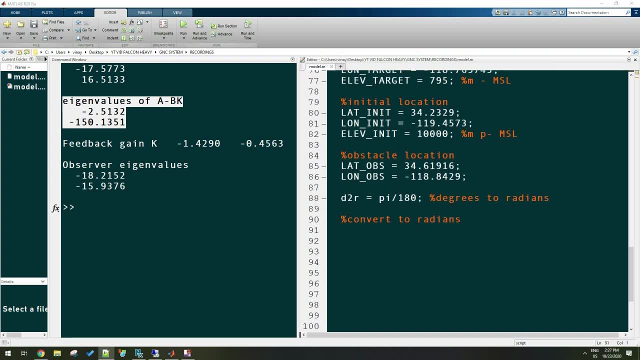 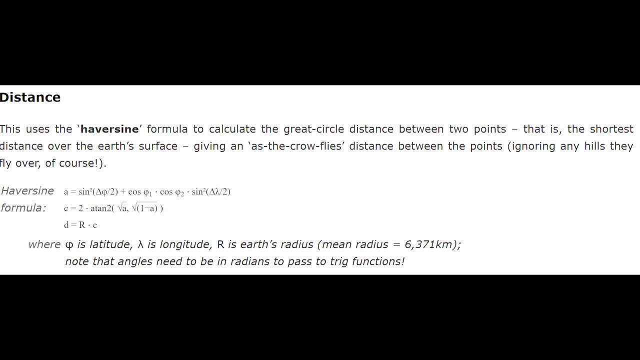 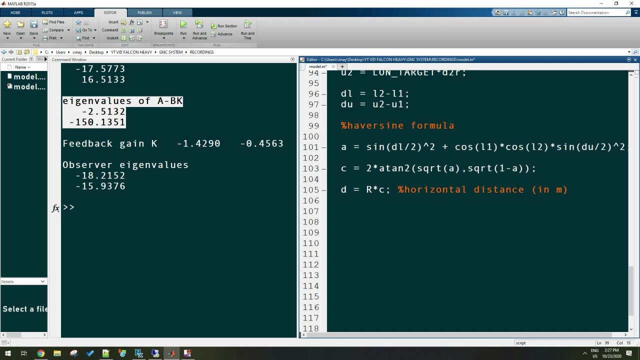 height, then the location of the obstacle, and degrees, latitude and longitude. we have to go to radians to use the math lab commands. so now we are going to use the Haverst Alice formula to calculate the distance between the two latitudes and longitudes. this formula is standard. okay, you can just Google it. so just plug in the values there. 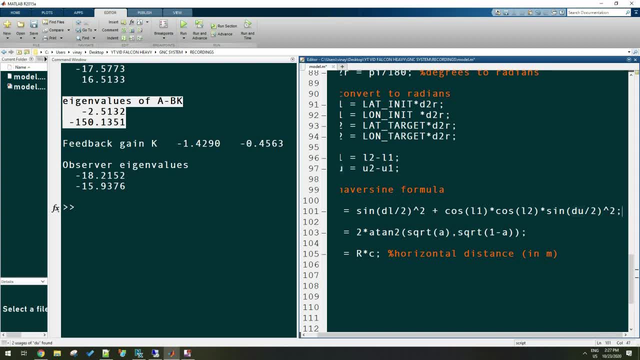 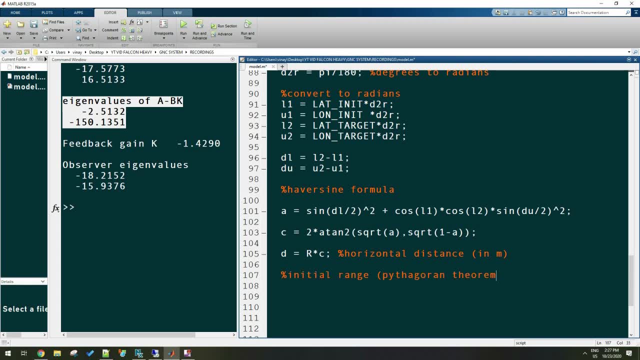 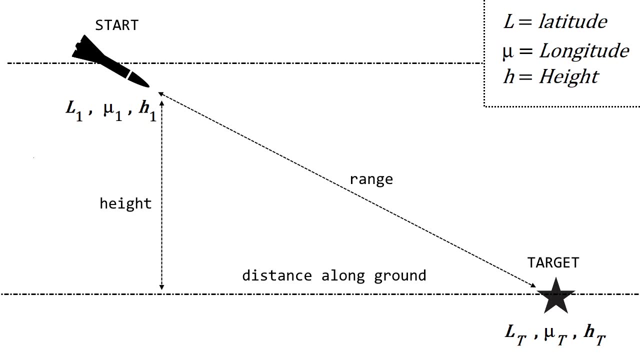 and you can get the distance there very easily. so this is the distance across the floor. it's not the range, so you have to separately calculate the range by using the law. so that's just square rooting things. so just do the left target minus 11 it. 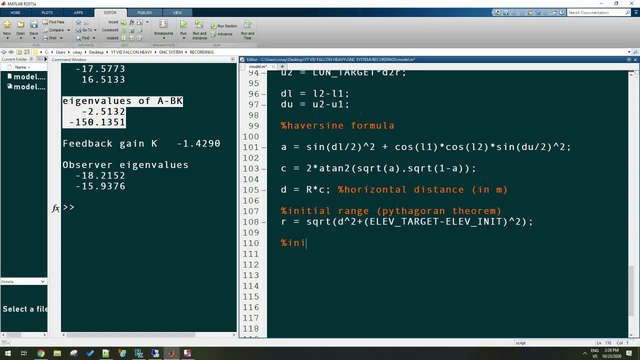 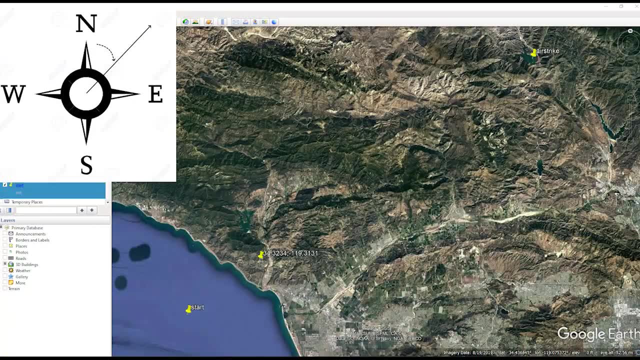 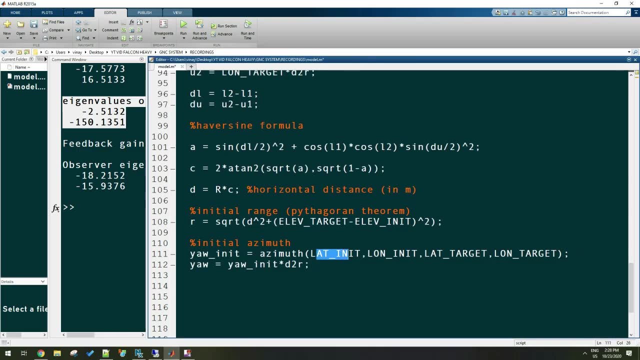 so you can see that there. then you can calculate the azimuth angle by using the MATLAB azimuth command. Azimuth is the degrees clockwise from north between the source and the target. so it's about 52 degrees here. so you can just do it here, as you can see there. 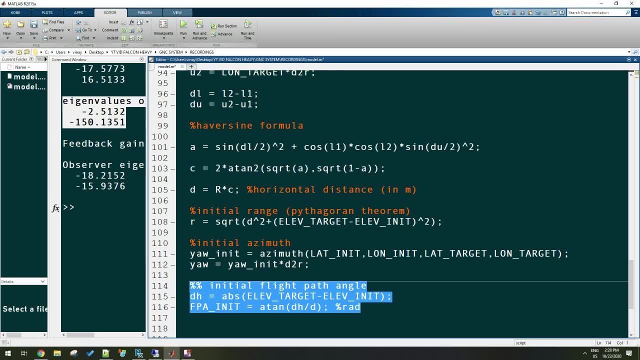 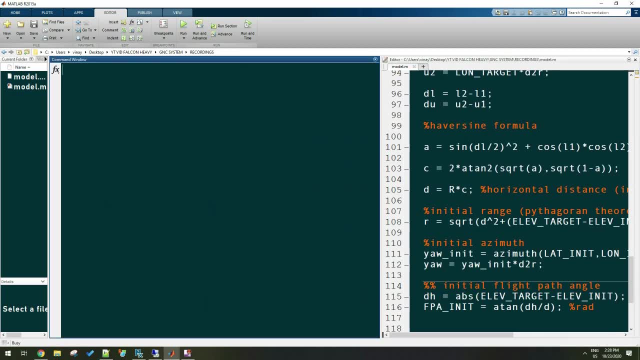 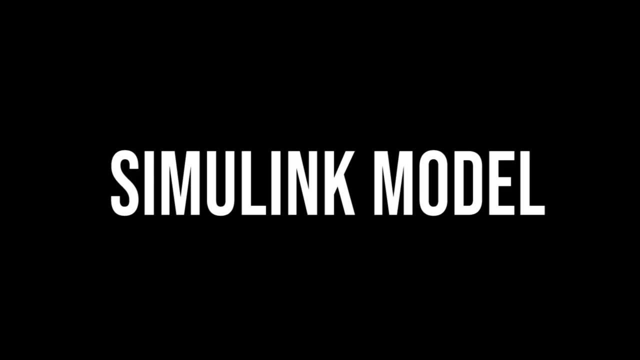 so that's the yaw angle which you have to maintain. lastly, you can calculate the initial flight path angle which you need to be at, so then you can run the program and the initial angle is about 0.11 rad. so it's not that much. Let's begin with the Simulink model. we have to first define the 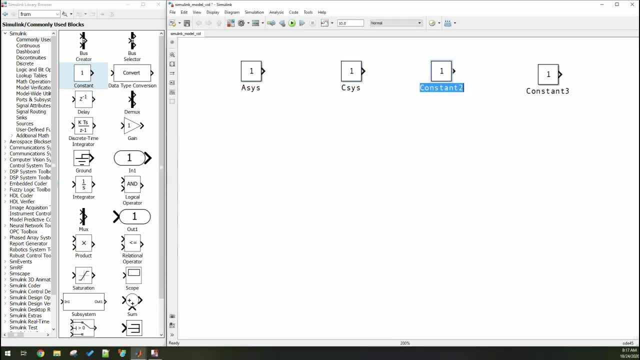 matrices ABCD once again, because they will be dragged in from the MATLAB workspace. so just drag in the constants there and define it as you can see I'm doing here. you also have to define, obviously, the LQR matrix K and, along with the observer matrix L for the Kalman filter. so just do that. here you can drag in the. 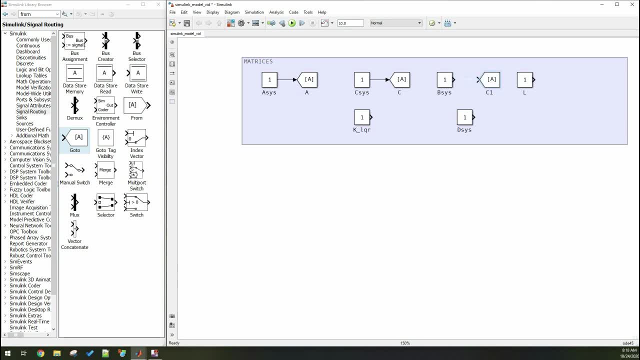 go to block, to make sure that you can then make it look much nicer in the model itself by using the from. so this I showed in my video: the MIMO Kalman filter design. so just define everything there and then you can start to build a model for the. 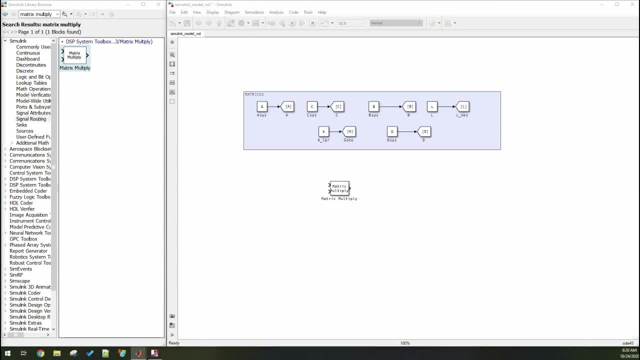 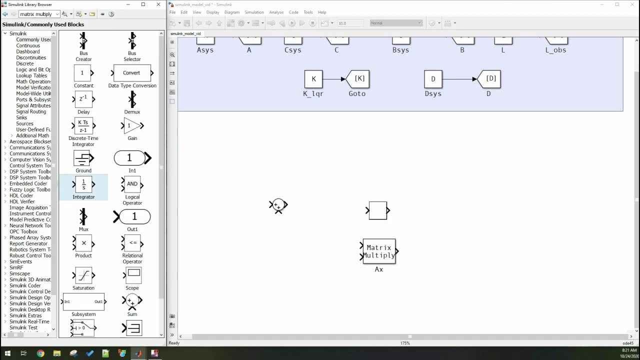 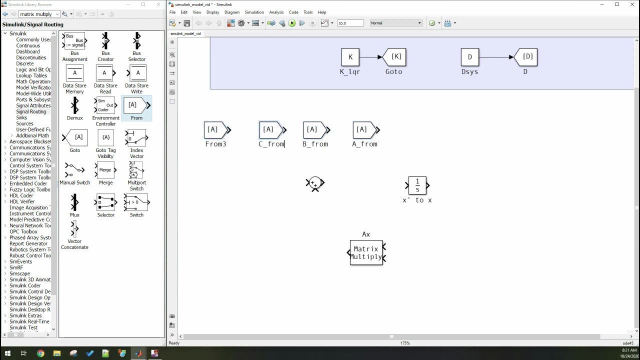 style and the filter as well. so let's use the matrix multiply block to accomplish this. so we have AX there dragging the sum. so X dot to X. so we take the integration of that and drag in the from block. so this is. it is bringing from ABC and D, so once again we have X. 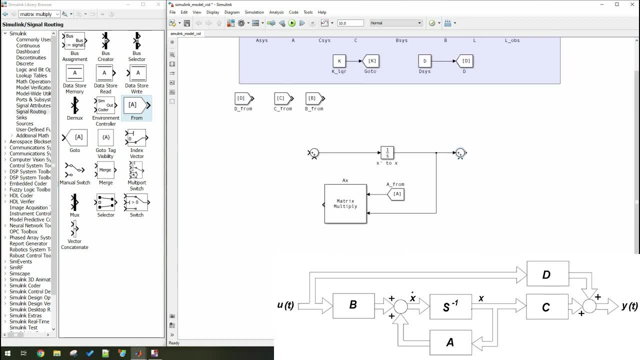 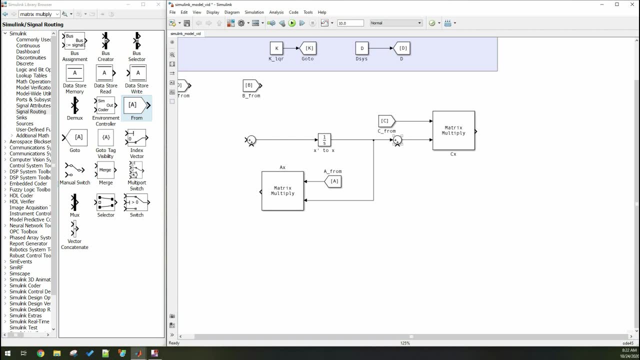 dot equals AX plus BU, just as normal state space model. there we have Y equals CX plus DU, so I'm doing Y right now, and then we have the feed forward term DU. so D times U- that's the input there- B times you. so disrespect once again. and we have you there as the sings single actuator. so we have D times. 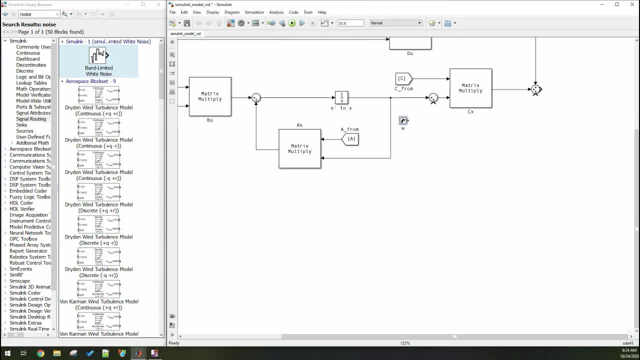 you. so that's why there. then we can drag in some nice w, so that's Y, while and out we have X, T, so that's y. there also we can drag in that Modว in charge of Y times U. and now come back to the semiatica and I see they fnc value for the base of X, so we're not able to modify them. so that makes me wanna change that and we start on that. and then let's talk about the eq 4xl. say your final infoc points, so facilities, we can connect parking for a fix unit type city in the eq4. Apache Oercaseь Englishxis우�. scream call from the eq eq4 or a free window, and then you can use some sort of 2015 понятно. 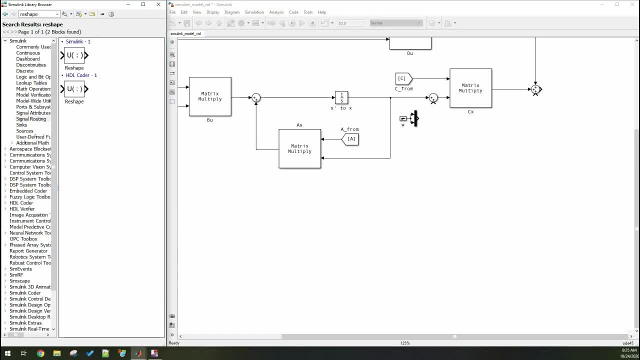 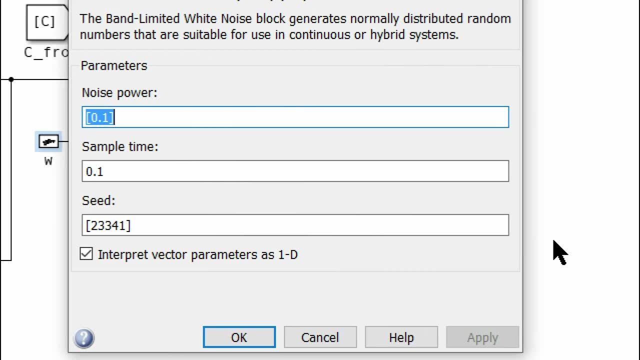 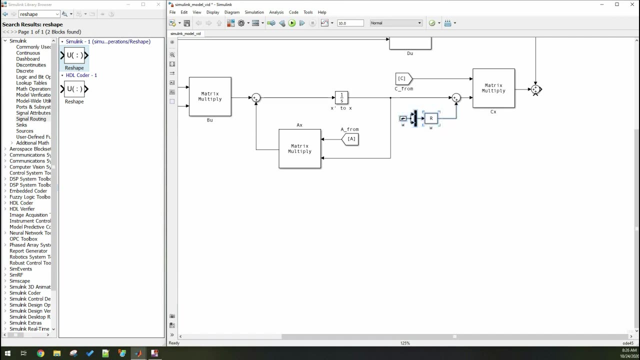 so that's for the process model, that's the x term. reshape that into a two by one matrix or an array and then assign dt1 as the sample time which we defined in the MATLAB model before. so copy and paste that for y, because we have cx plus v, this is v here. so that's the noise for the. 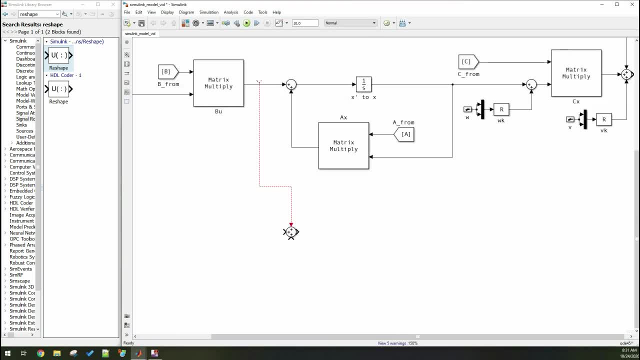 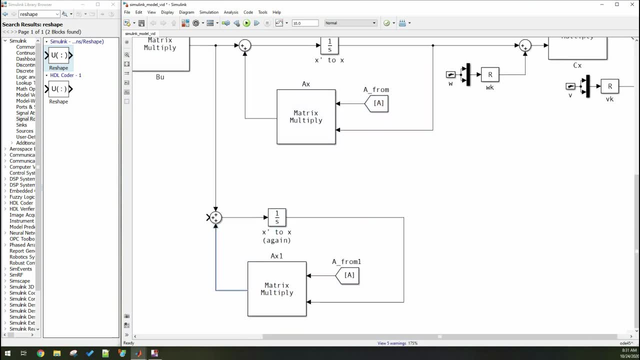 measurement and once again we can design our common filter. it'll just be a copy of the system, so it is simply x hat, because x hat is the estimate of x, it'll be: x hat equals ax plus bu plus l, multiplied by y minus cx minus du, and you will see what i'm doing here. it'll represent that. 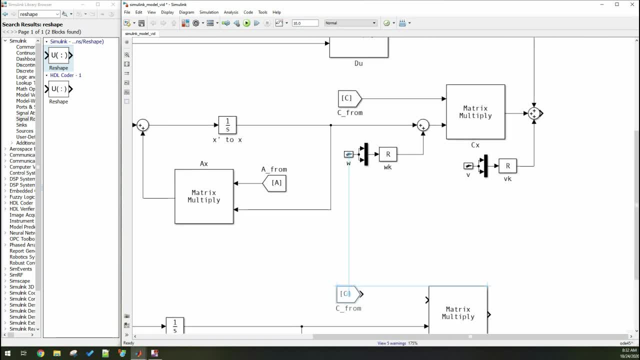 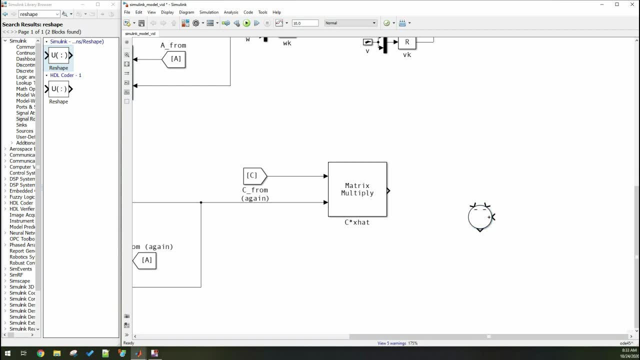 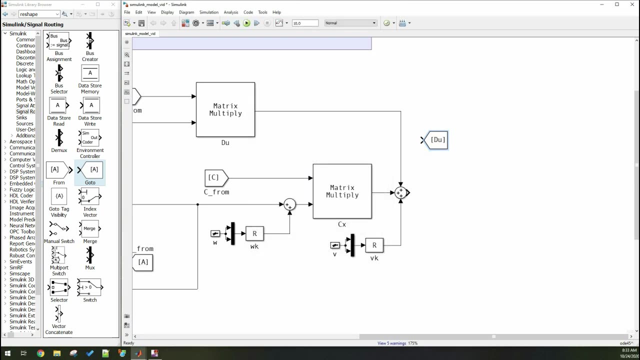 so so that's our x hat there. so it's pretty much a copy of the system, right? because that's how an observer works. you so drag in the y there, but first we can just put a go-to block for the du term. it'll make our model. 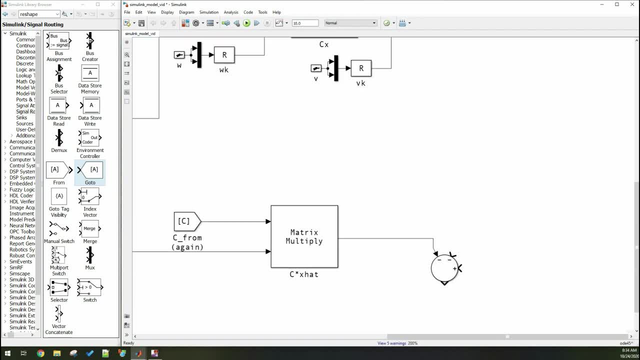 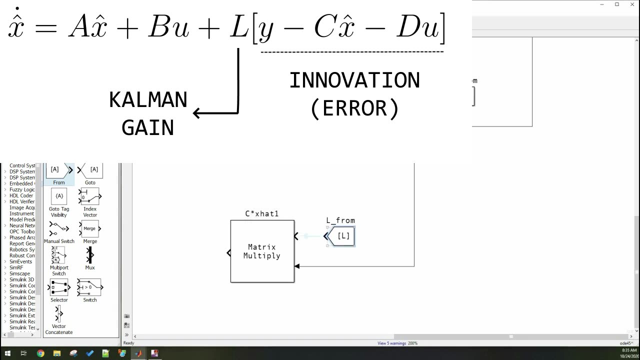 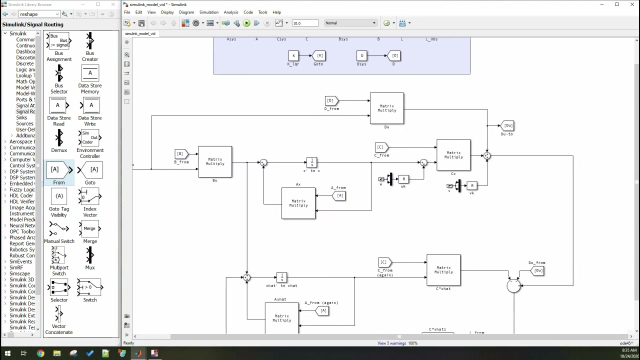 look more neater. so connect that to du and once again from du, so just adding it to that. so what we just did is y minus cx minus du, okay, and then we can connect that to the l, so it's l times y minus cx minus du. so that's our model with the filter. 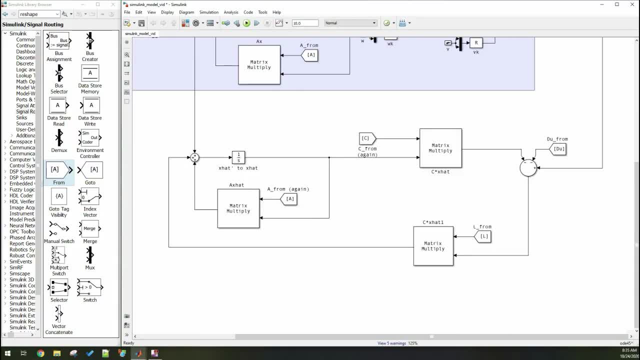 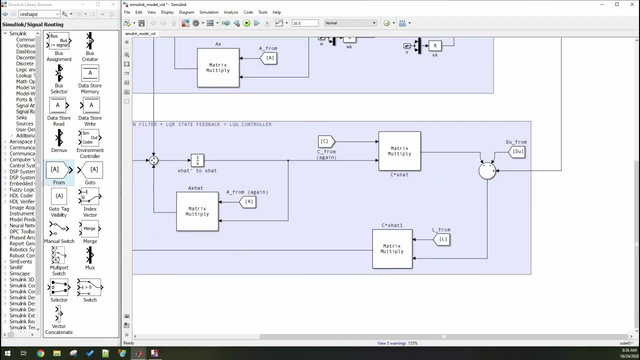 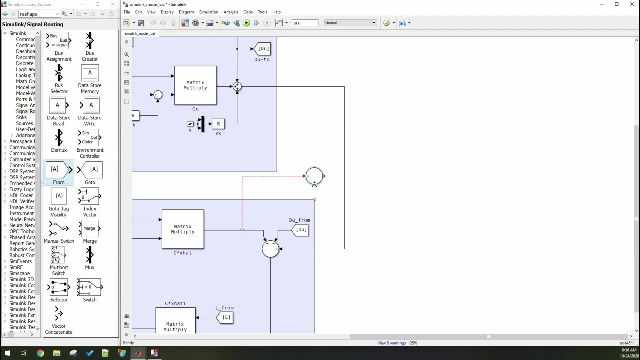 we can just put a block around it, define it as the filter. so that's the filter there. it looks um, it looks normal, i guess so, and we can do some connections here. we can extract some values from this simulink model. just remarkably useful, right? you can see that we have the same surfaces here. you can see that in a. 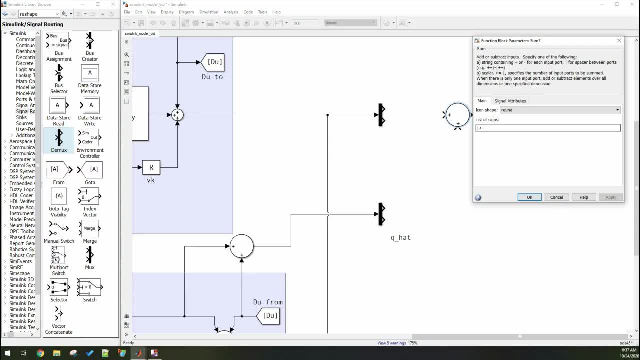 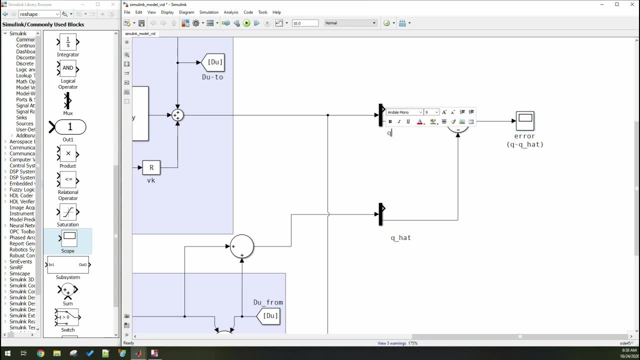 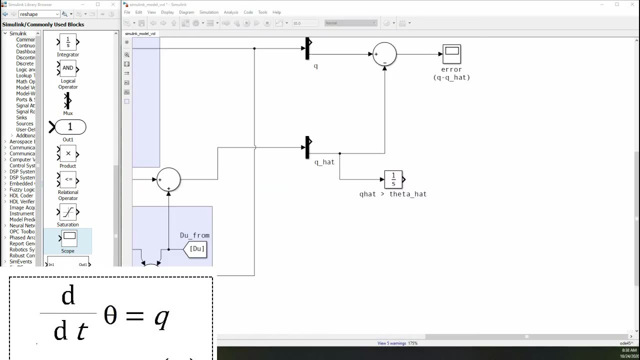 rilaxor actually, so you could demand that these filter's too big and this one here wouldesty. it's nice to be able to look, can't? we can use that as this? basically right, and now you can see that here we can order it under some parameters. exactly, this is the. 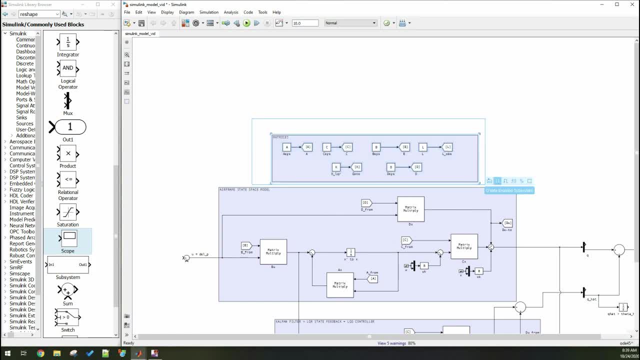 dimensional control that we're doing here. we can just templates, just for this savory pessoal, which you can then use as outputs. so that's q hat there, because that's a second state from the output. so at the second one. so we obviously have to do a theme multiplexer, you can calculate the error. so that's q minus q hat from the common filter and it has to be around zero. so from q we can get the angle by taking the integral of that. 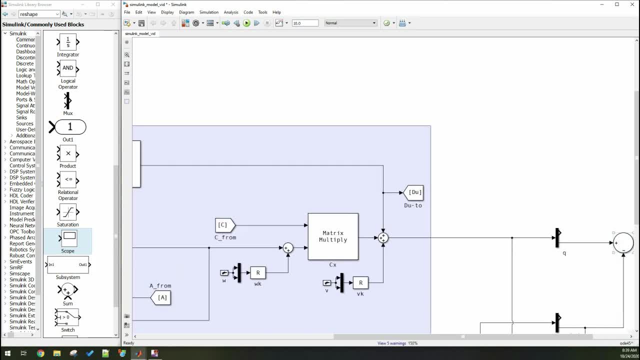 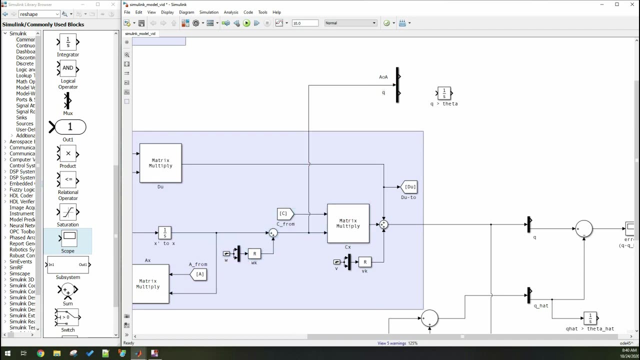 just move it around. we can also extract the states. so that is the angle of attack- AOA and Q- and we can once again extract the angle from Q. and i will show you guys, why i'm doing this. it is to build the guidance model which will be after. 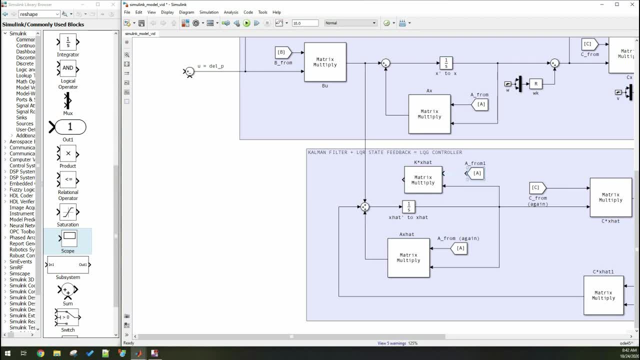 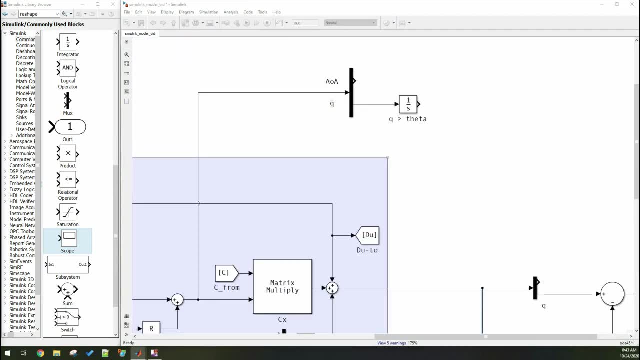 so we would need to obtain both Q and Q hat. so now we have the feedback gain, so that's the LQR controller there. so we have to connect that back into U, so it will be R minus KX, right? so that's what we're doing. 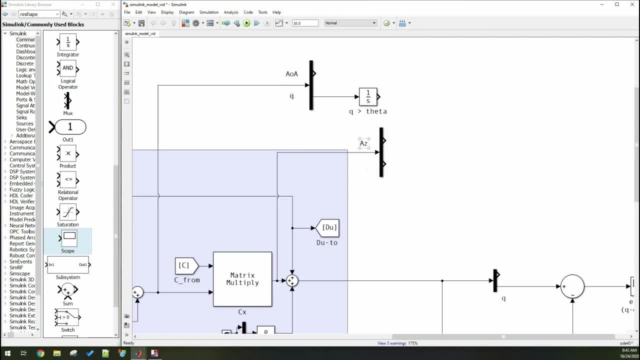 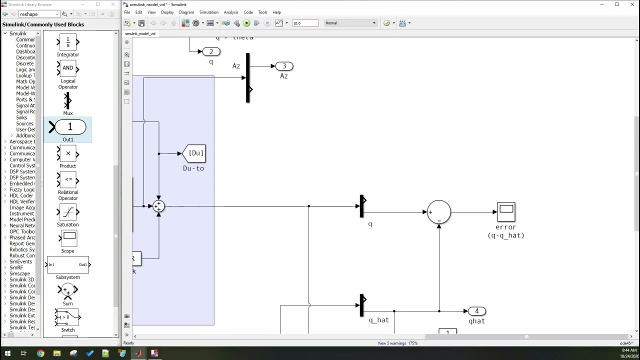 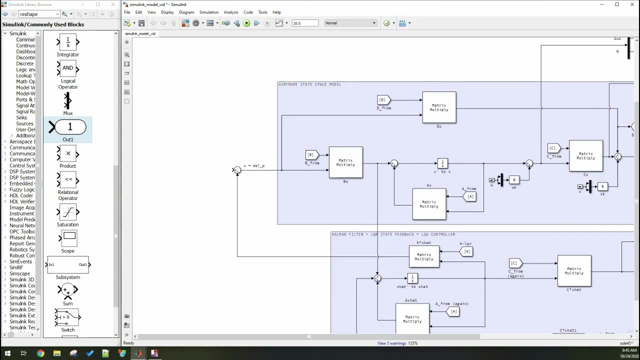 KX hat. i'm just extracting more values here. i'm extracting the actual outputs AZ and Q there, so that that's the from the Y equals CX plus DU expression. i'm just putting some output blocks so we can build our subsystem very neatly and it looks very neat. 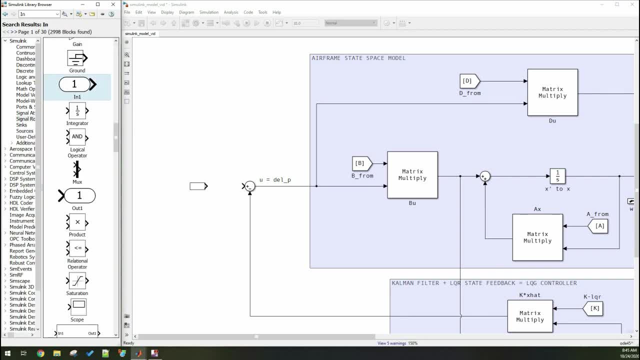 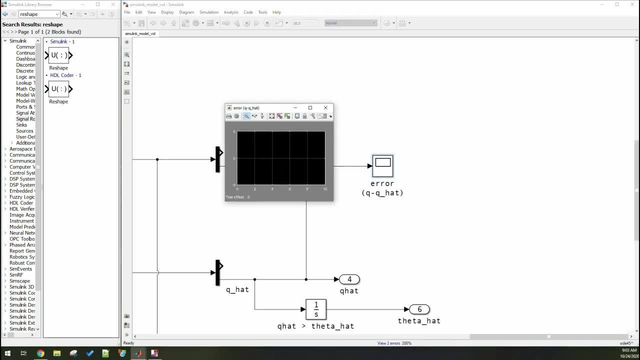 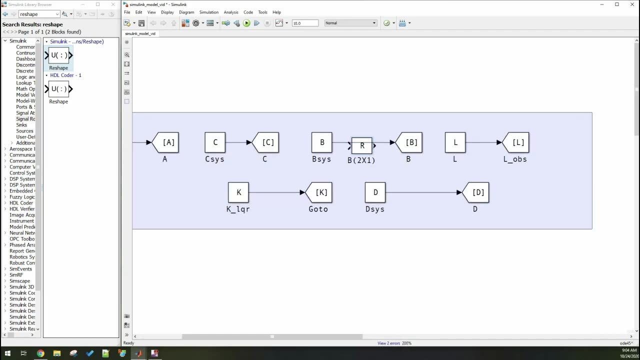 so then we can define our set point. so that's the desired Q, so the commanded Q, right, so that's our set point, so that's our model. there it looks pretty decent. we can just reshape these now, because otherwise you may get errors in matrix multiplication. you have to define an array as a matrix in Simulink, i think. 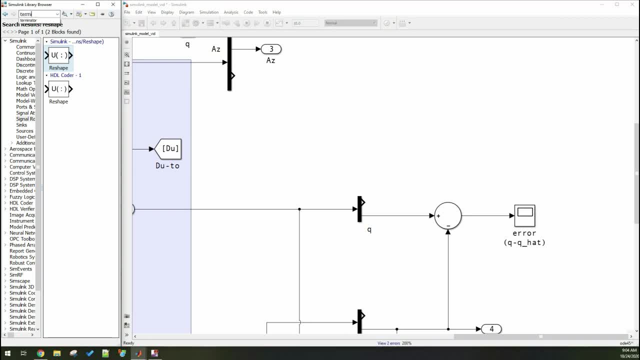 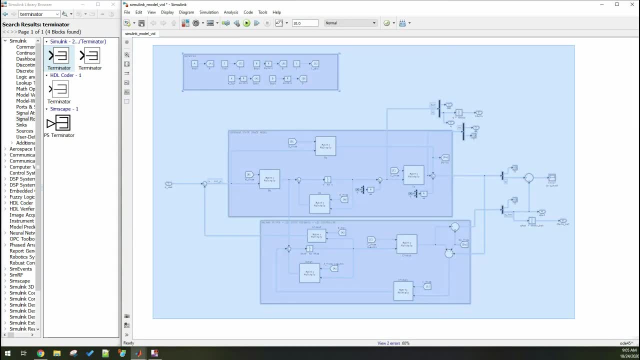 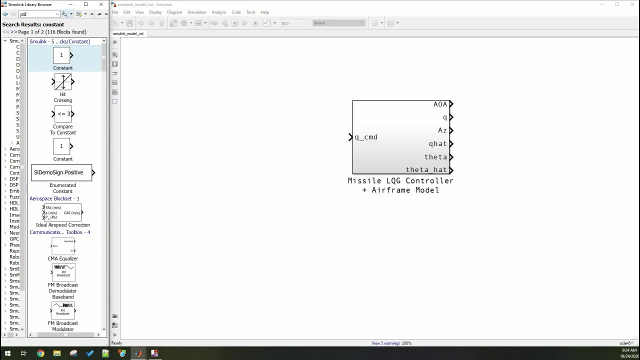 at least for me, i had to do that. so in my version of Matlab drag in some terminator blocks, because those will not be outputted, so they have to somehow not export. so drag a block and create a subsystem there. so that's our missile model with the LQG controller. 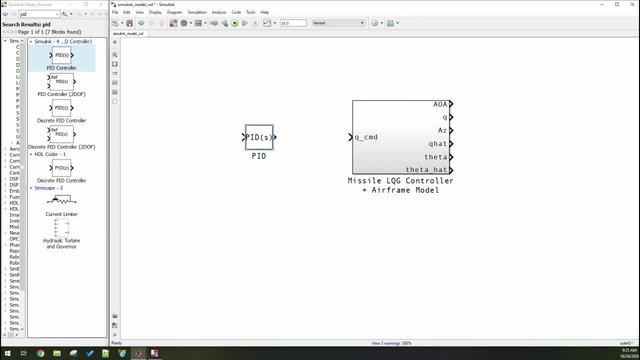 so that's our innermost loop and now we can define the second loop. so this will just put a negative 1 for proportional gain as a PID controller put a saturation because we don't want the commanded pitch rate to be too high because that will make the missile move too fast. 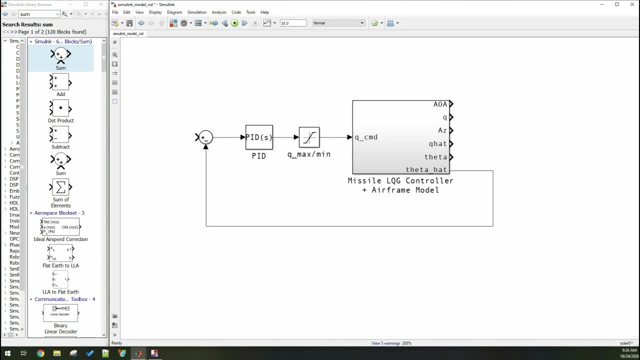 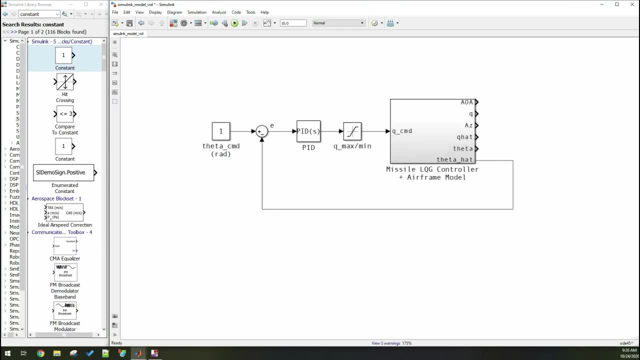 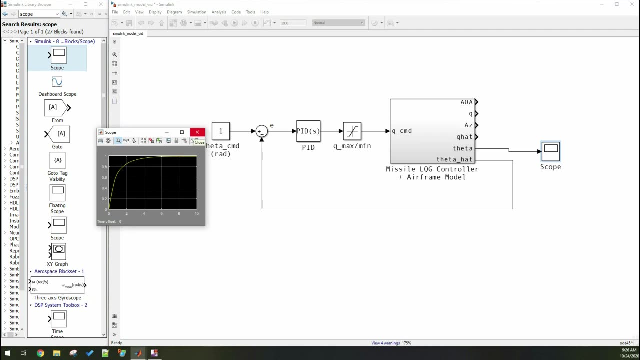 so now we are doing the outer loop and we connect the estimated pitch angle and we can define our commanded pitch angle there. so we have this going on. this is a two loop control system. let's drag in a scope and do a run so it tracks. well, it achieves 1, so that's good. 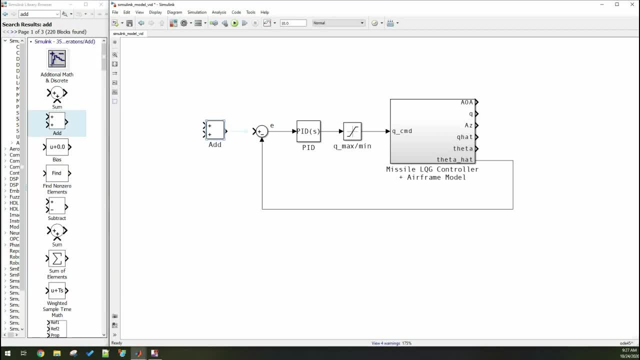 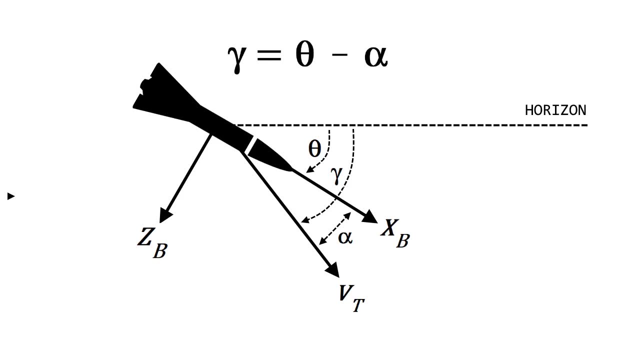 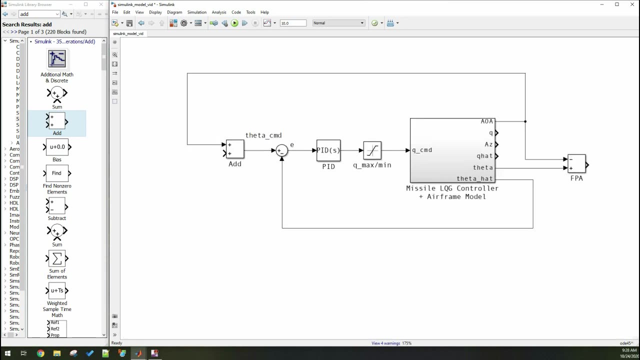 so we can now do it for the flight path angle which we need, and from the expression you can then extract the commanded pitch rate from the angle of attack. so just calculate the flight path angle here from pitch angle and the angle of attack once again. so you have to assign the commanded flight path angle there. 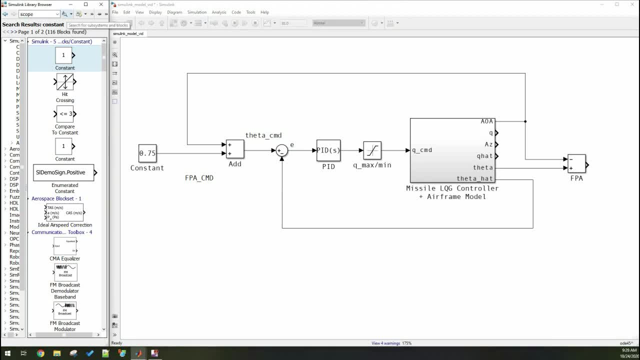 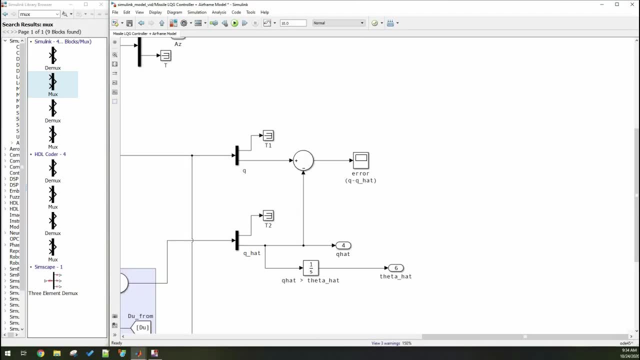 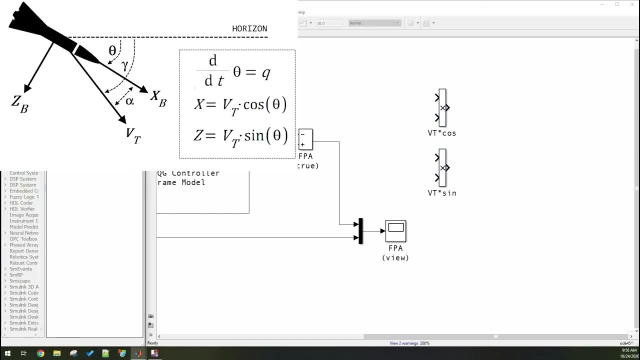 and if we run this one here, but first we can drag in a scope to make sure we know what that looks like. so it tracks well again, right, so that's good. error is 0, so that's also good. now we can define the guidance model, so that'll be x and z. 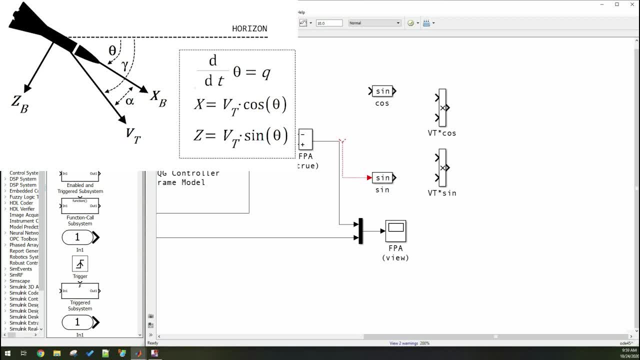 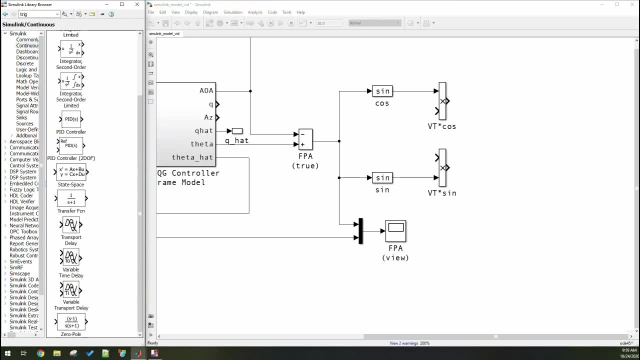 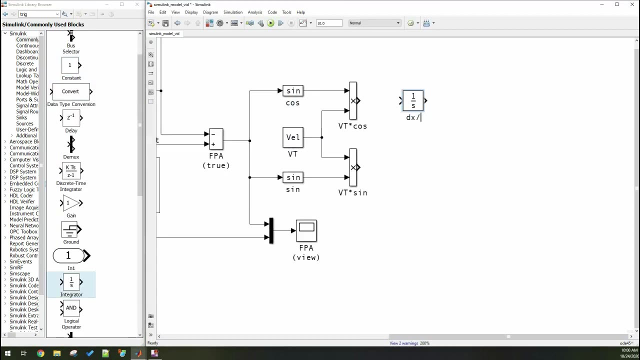 so obviously x equals velocity times cosine and z equals velocity times sine, as you can see there. so just define that here. velocity is a constant, so we can drag in a constant block and assign it to vel. that's the variable we used in matlab, so we have to use that one. 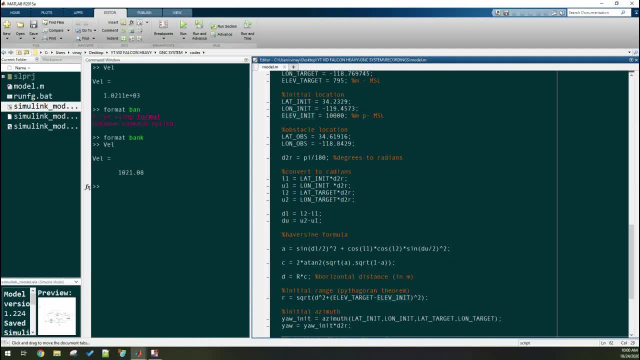 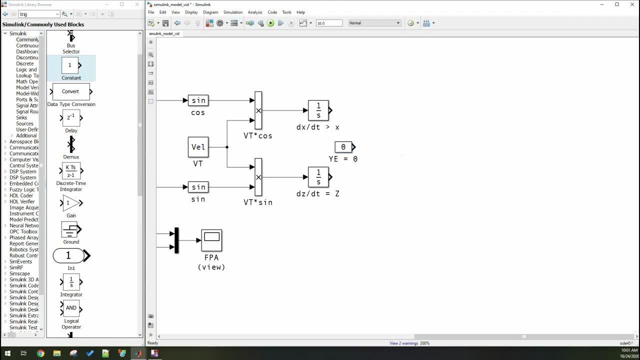 use an integrator block once again to extract. and now is z initial equals elevation in it, because it starts at a height. y equals zero because we don't have any y there. it's only in two dimensions for this example. so that's our x, y and z position in meters. 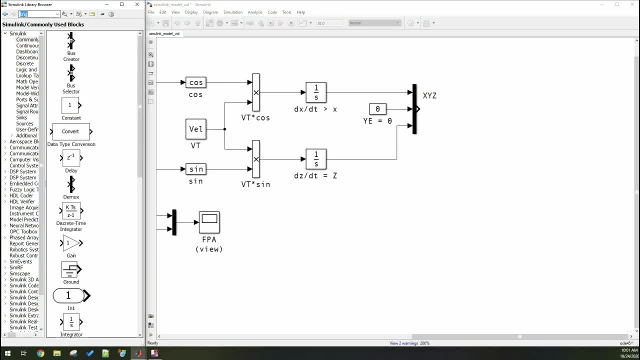 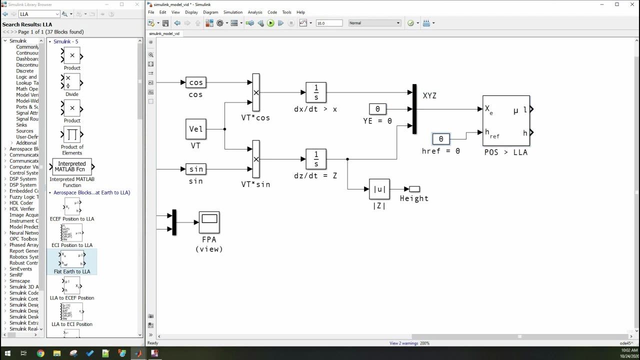 you can define the absolute value of z and that that's your height. so this block here, the flat earth to lla, converts position to latitude and longitude and altitude. so that's lla. so we have to use that block. this is in the aerospace block set if you don't have. 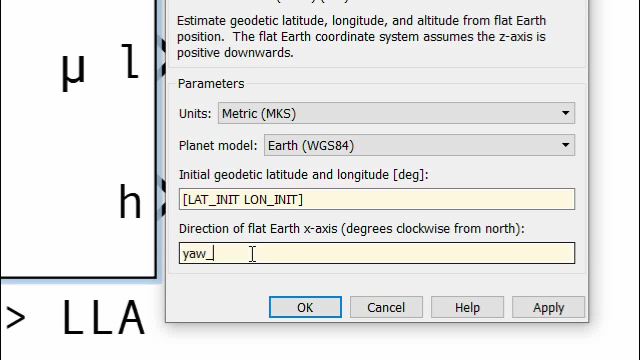 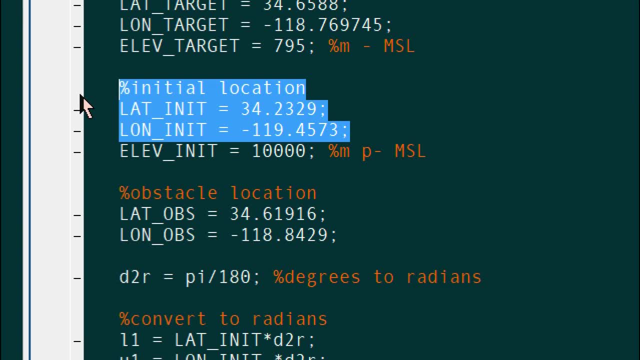 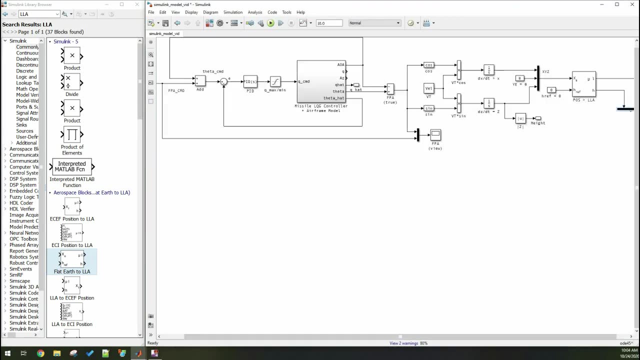 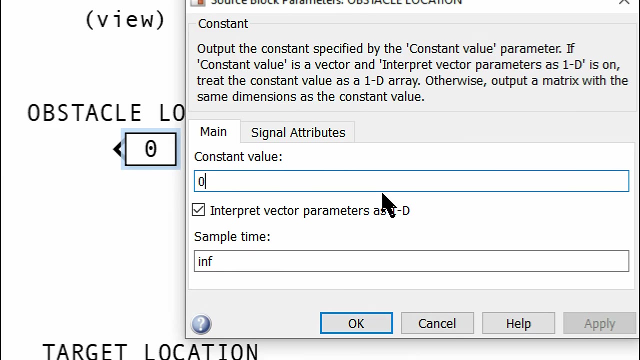 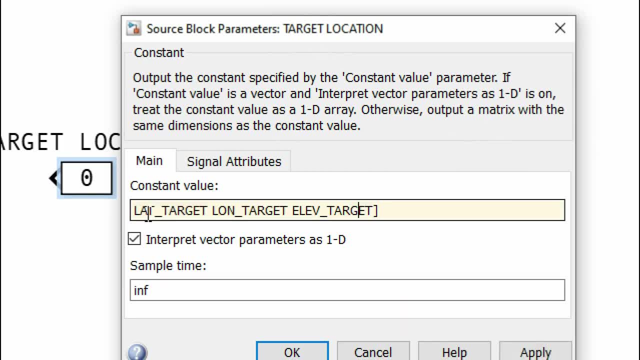 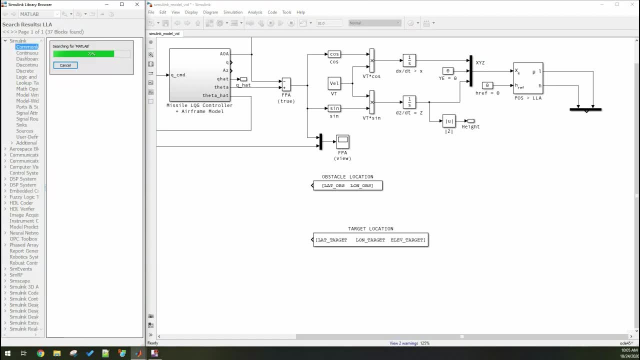 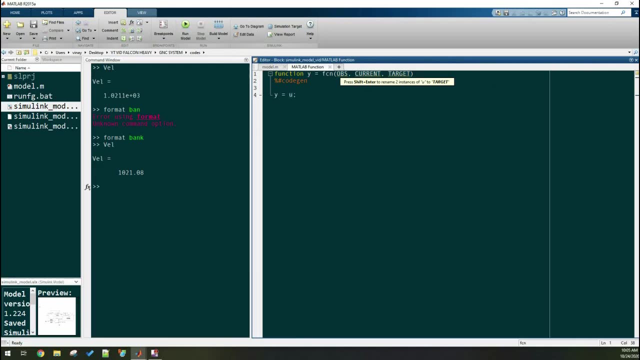 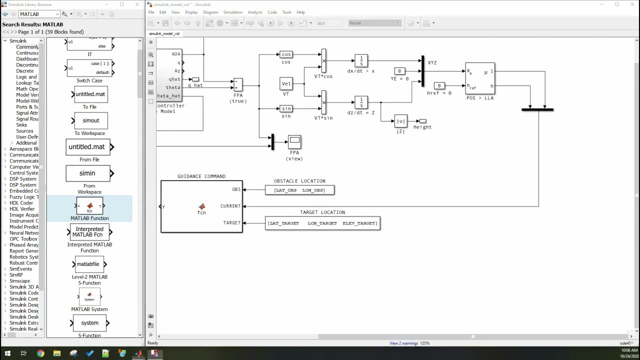 and we can drag in a matlab function to do the calculation for us. so let's just do that now, so it'll take in obstacle, current and target locations and you just connect the blocks there. that's the guidance calculator and we can also show the location with the display block. 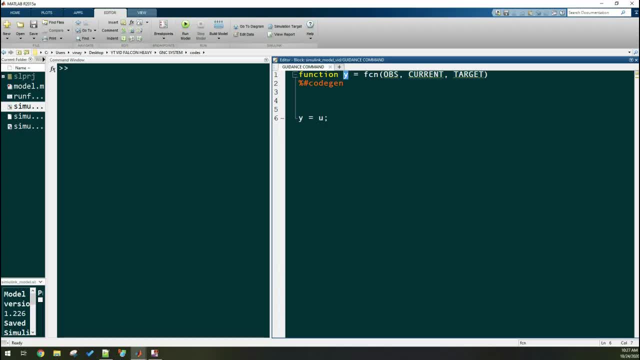 so let's define what we need to calculate. so we have flight path, angle range, distance to obstacle, altitude and the warning command. so let's define the same stuff we did before. so obstacle location, obstacle zone. so that's the no fly zone, target location, current location, distance to target from the obstacle. 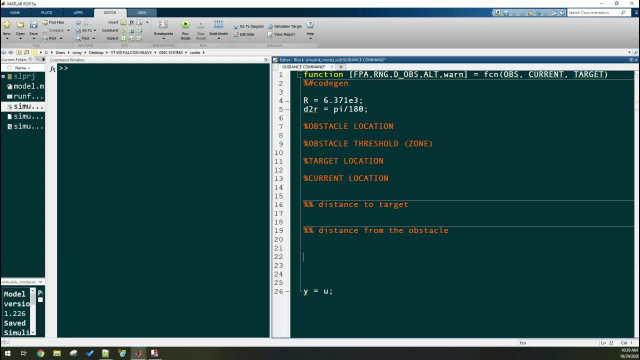 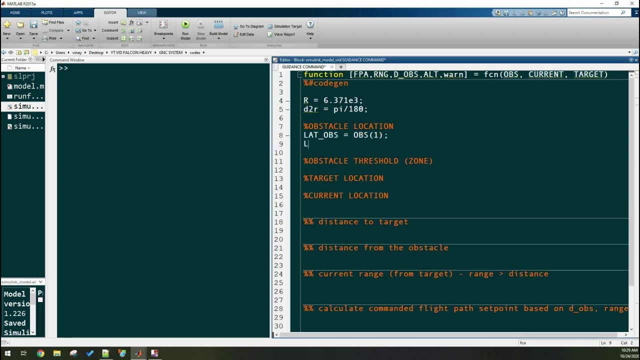 the range from the target so and the flight path angle, based on all these values. so this will be very interesting and you'll see how i do it here. so first let's extract the locations we need. so we have a two kilometer zone there, so that's your no fly zone. 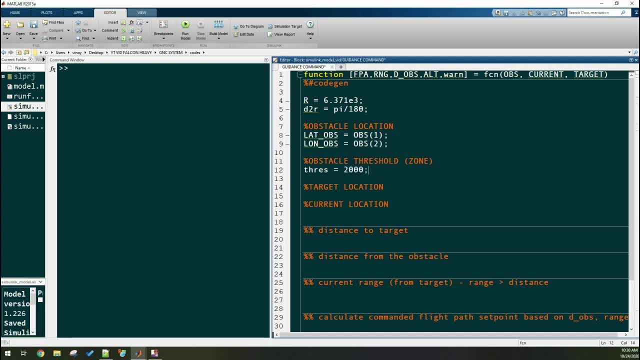 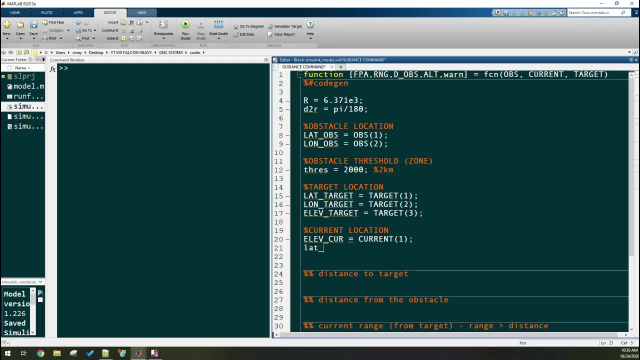 we have the elevation, the latitude and the longitude of our current location. it's in meters and our young point between that point and that point is the exit point. so this is the No Fly zone. so we'll simply gone for the basic initiative and hitting the stop button. 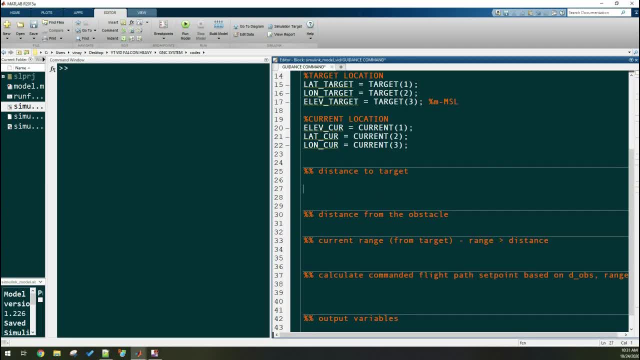 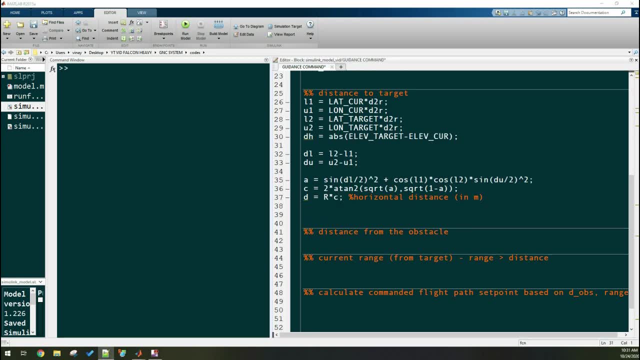 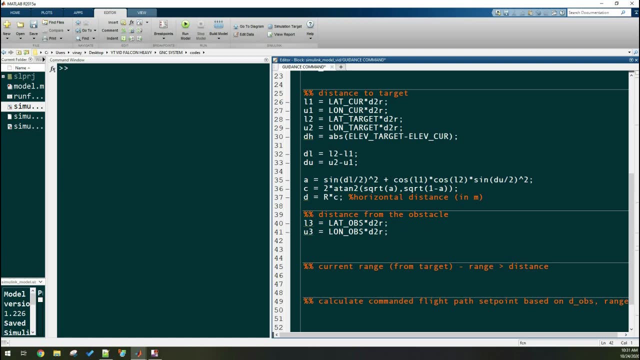 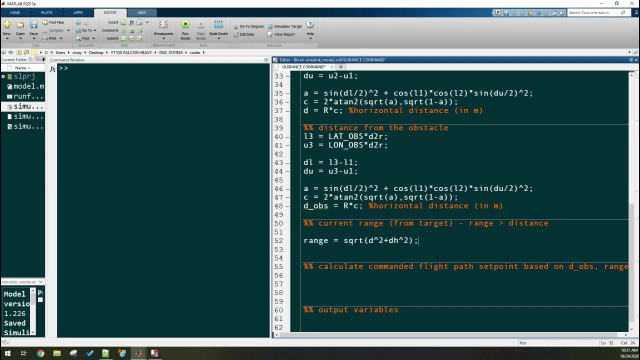 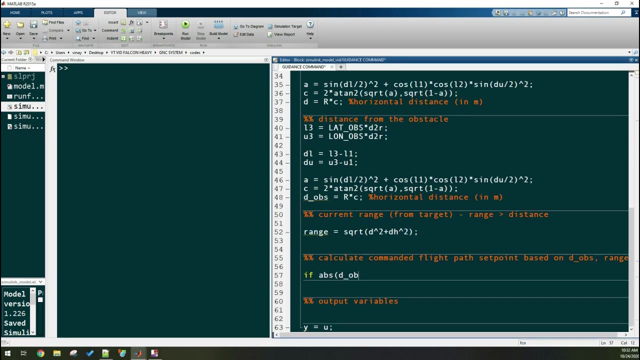 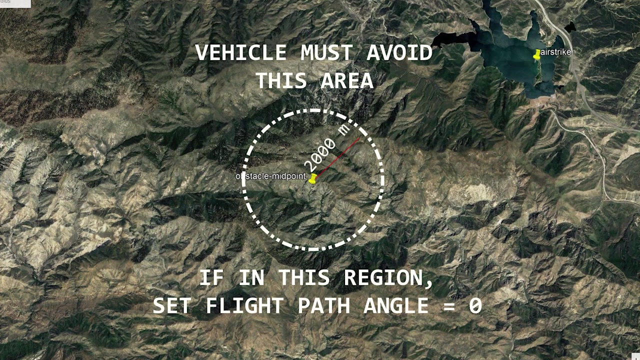 so it'll show me that and i'll. simplyagement two: let's again use the centimeters here. range from the target. So to calculate the flight path angle, the command is very simple: If the location from the obstacle is lower than the 2000km, you make the flight path angle. 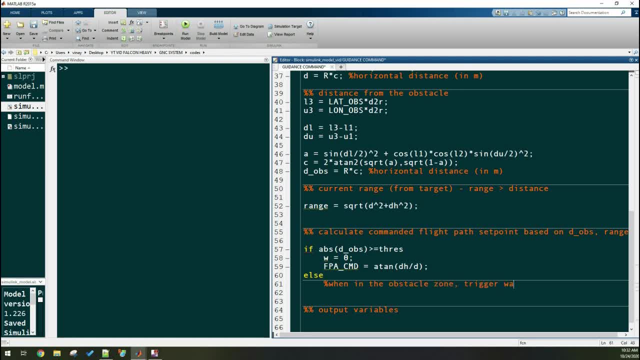 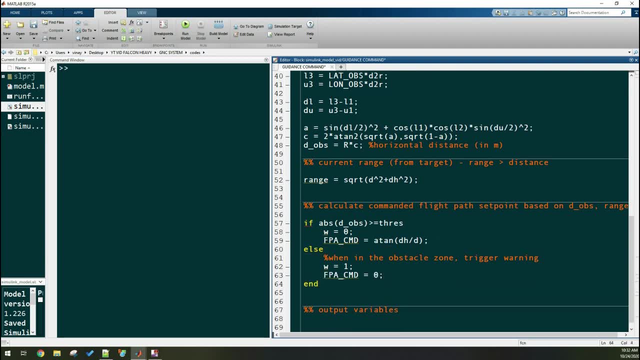 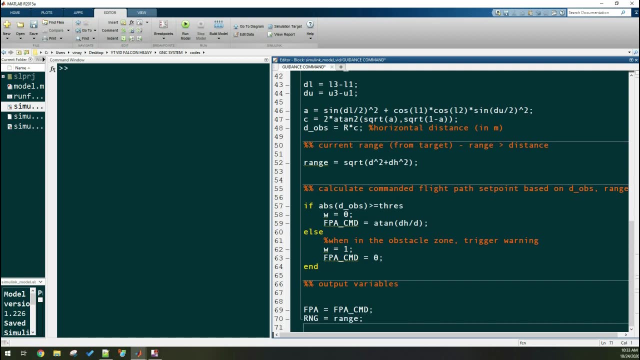 zero and otherwise it will be just the arctangent. So it's a simple command. So here you can see I'm using an if-else statement. I'm sure this is what the aerospace vehicles use as well, like on their machines. Now we can set the output variables. 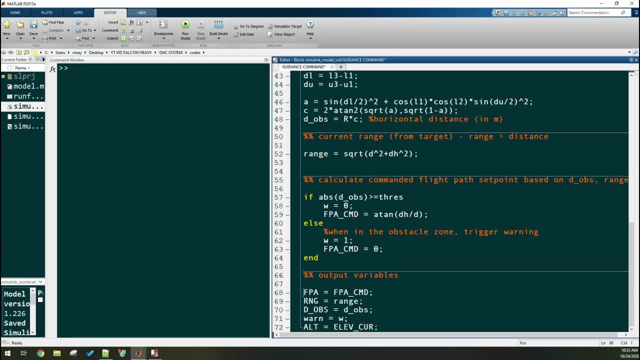 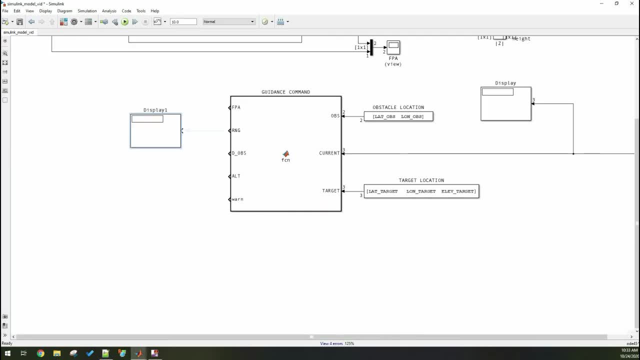 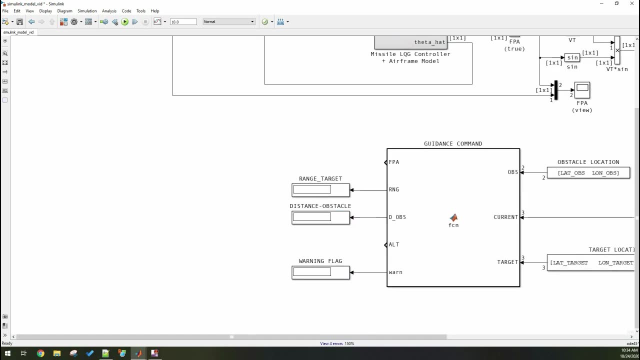 You set the flight path angle, the range, the obstacle distance, the warning and the altitude. We can feedback the flight path angle, But first we can display it, So we have some stuff that we want to see. so the target range, the distance to the obstacle. 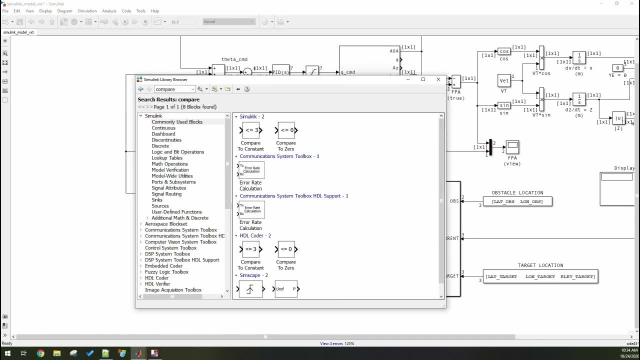 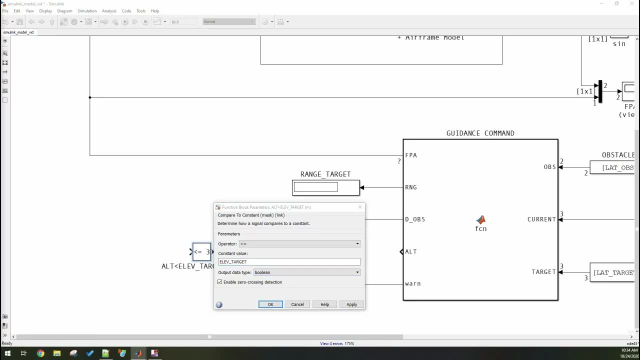 the warning flag and just connect the flight path angle there. So, lastly, we can just when the missile height is lower than the elevation target, so the target height. that's when you can stop the simulation. So you can do this by using compare to constant and then using a stop block to stop it. 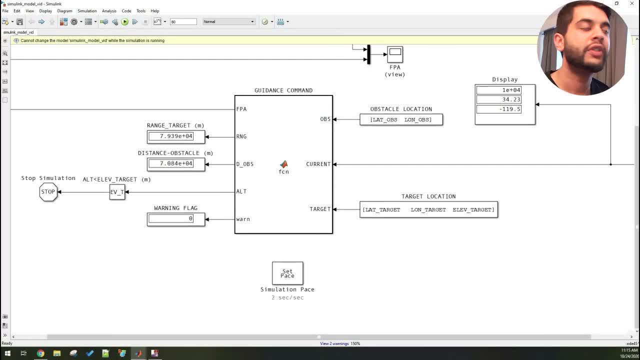 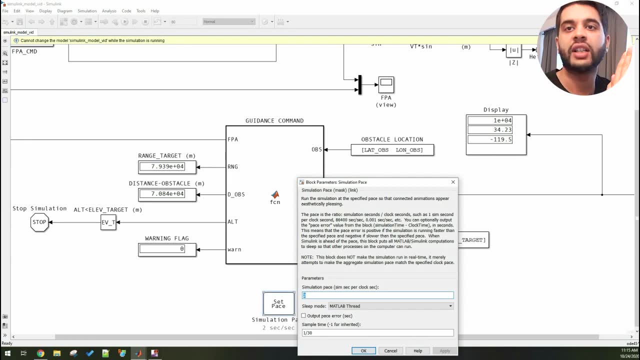 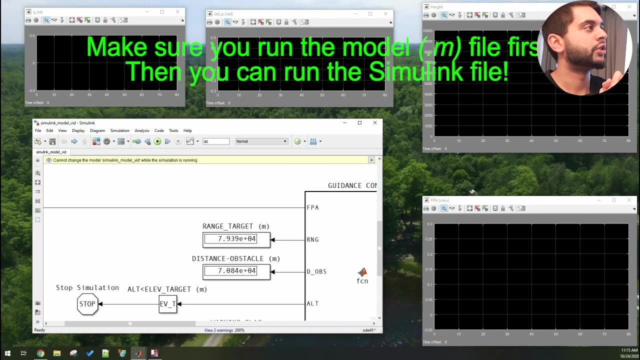 So we have the simulation done here And if you take a look at the model itself, You have the complete guidance, navigation and control system built into one whole simulink model and that is called an integrated system. This is what we do and I can also run it now, so make sure you first run the MATLAB file. 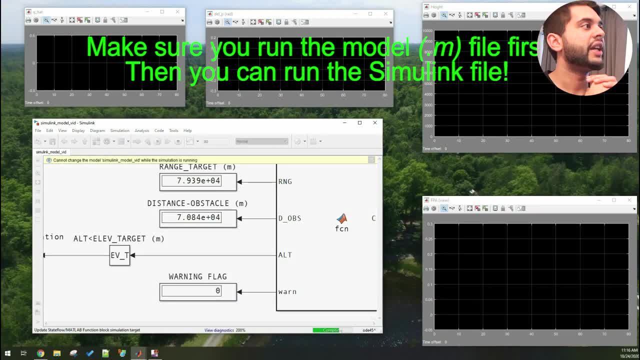 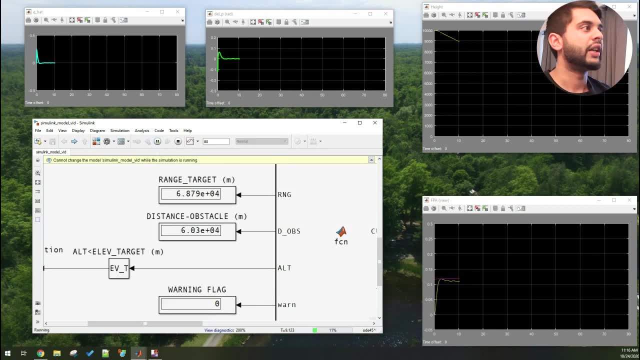 and let's compile it first and then let's play it. So when you play it you will see the range from the target go all the way down, because obviously it's getting closer to the target and the distance to the obstacle is also going down. 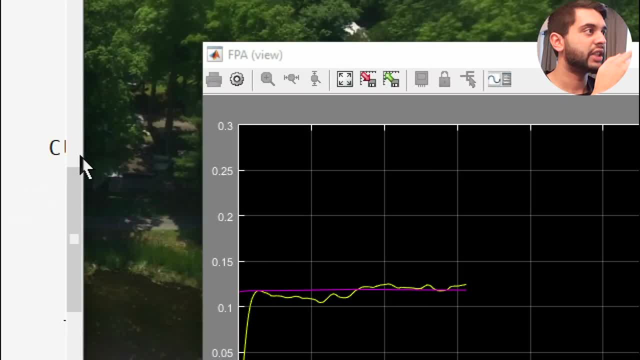 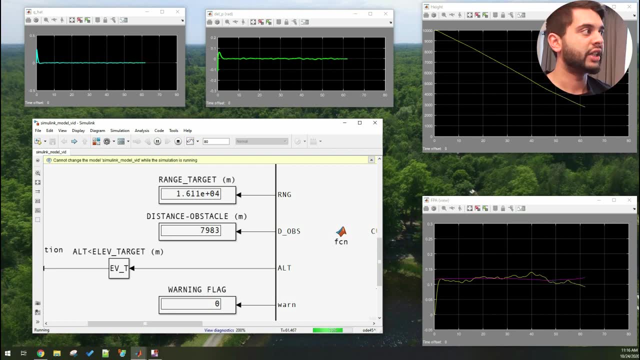 The height is going down there, as you can see. The flight path angle goes down there and the moment it gets below 2000 meters from the obstacle, the flight path angle will change, As you can just see there it will become zero and then it will get back to where it is. 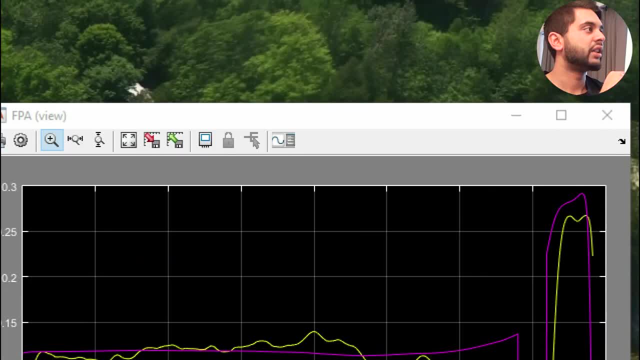 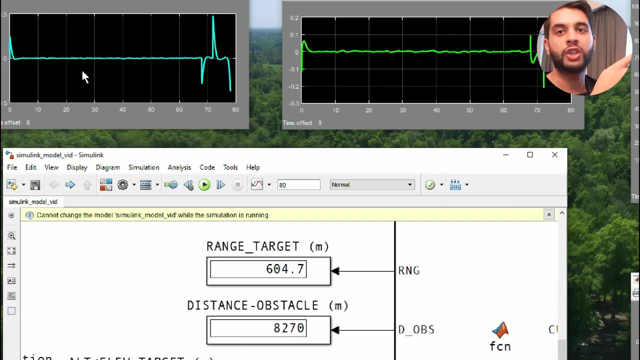 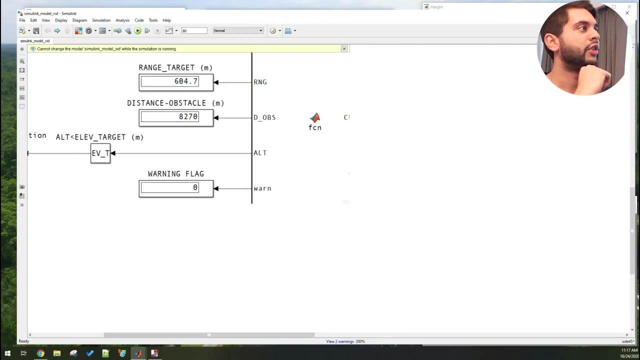 So that's the flight path angle: getting zero there. That's the obstacle. at 70 seconds it will reach it and it will avoid it. So, lastly, you have the pitch rate there commanded so it does not exceed 1.. It is the actuator input, so it's quite good performance. 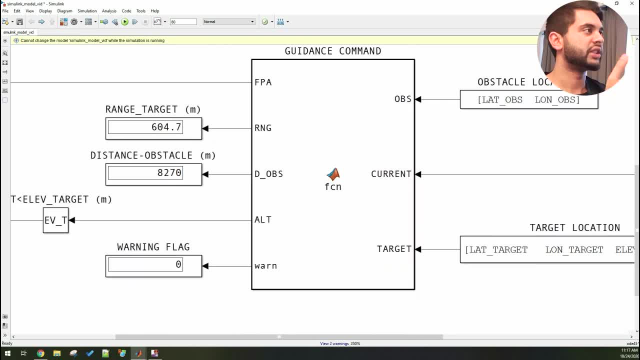 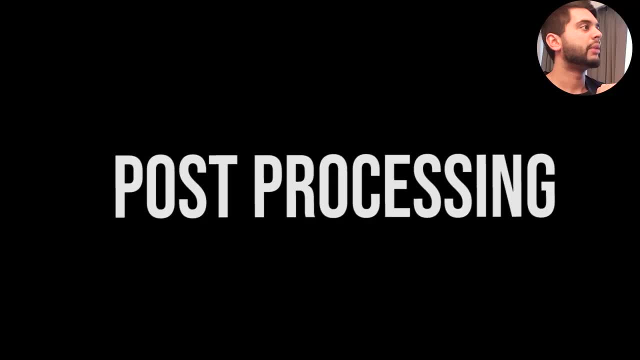 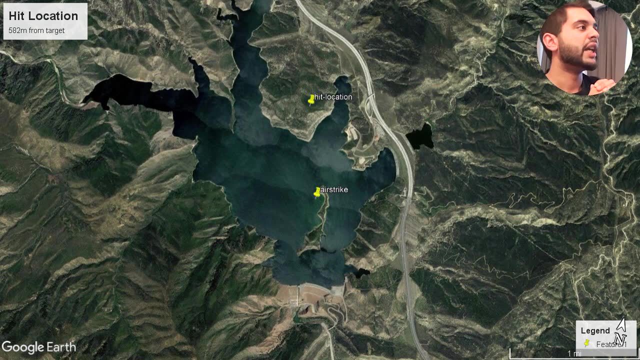 It's about 600 meters so it does miss, obviously because you have noise in the system. That's the final location. If we google the final location on google earth, we can plot it. so it is a bit far from the target. it does miss a little bit and what they do is you have to plot a blast zone. so 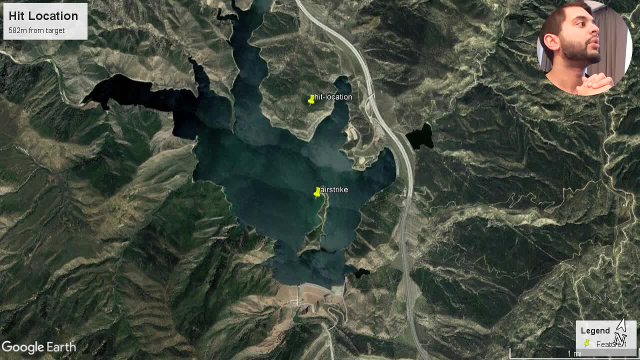 if we first go to a location and if we plot a circle around it, and the same for the target. as you can see here, You can quickly compare the accuracy. How the blast accuracy is calculated is simply: you take two zones and you find the common. 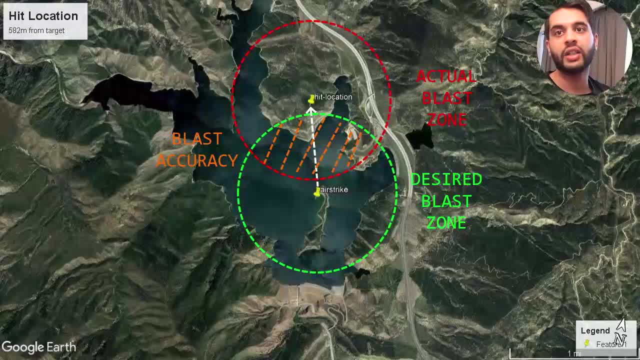 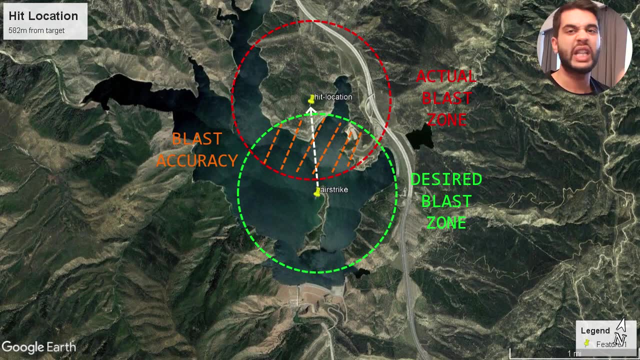 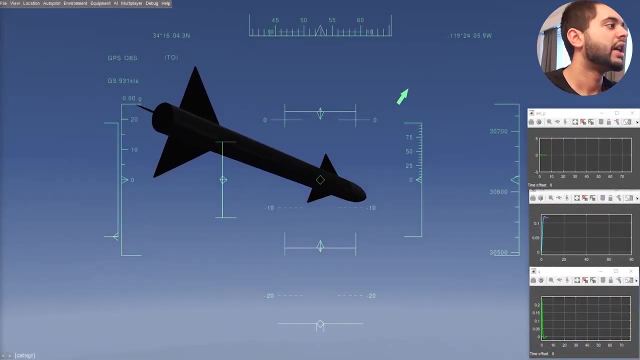 area. so that's here, and you divide it by the circle area. so We can now do this in flight gear, as I did here, and I have many videos on how to use MATLAB with flight gear so you can take a look here. You can see how you have the missile in the air is going all the way down and I'm playing. 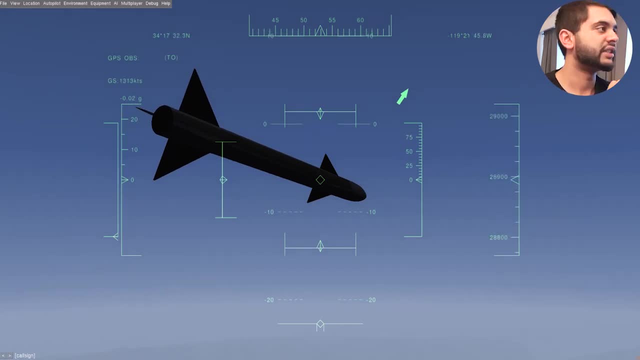 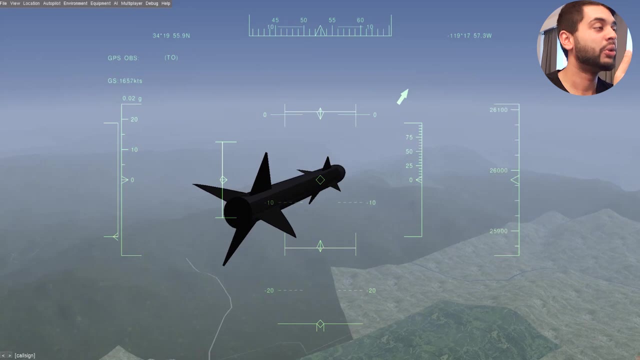 the whole simulation just to show you what it looks like. so it's descending at a flight path angle all the way down. It looks so awesome like. when I saw this I'm like, oh my god, this is so cool, I'm actually doing a real-time simulation and it's almost like I'm working at some top. 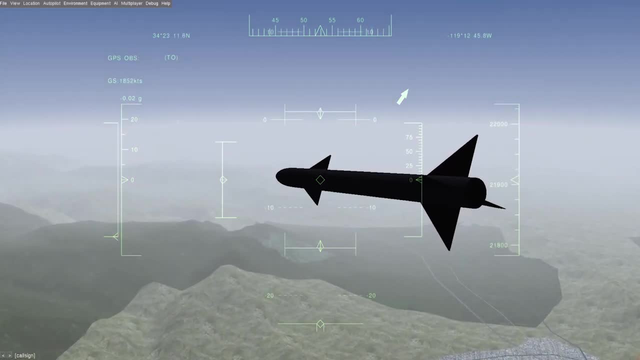 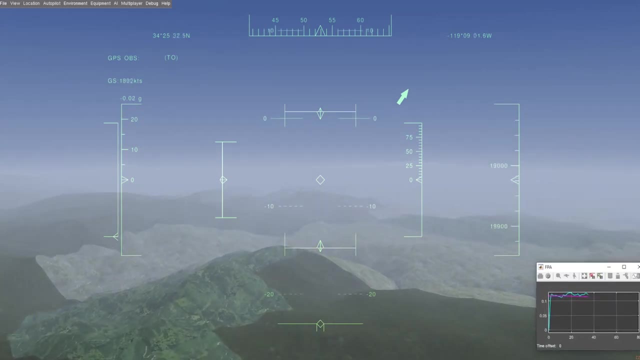 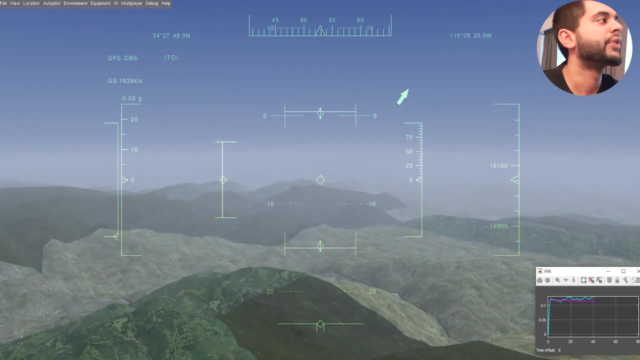 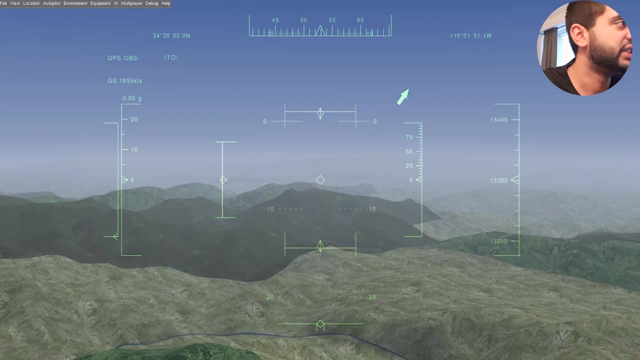 secret lab at, like, I don't know, Northrop somewhere, and you can also do this yourself. so you can see how the obstacle is coming up. it's the mountain up ahead there where the Target pointing to. so it's descending, descending, descending. it'll reach the mountain almost. 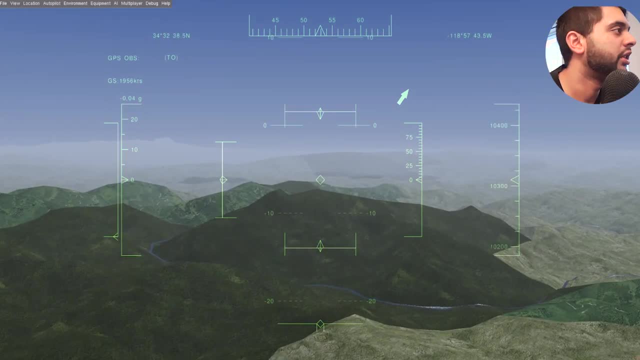 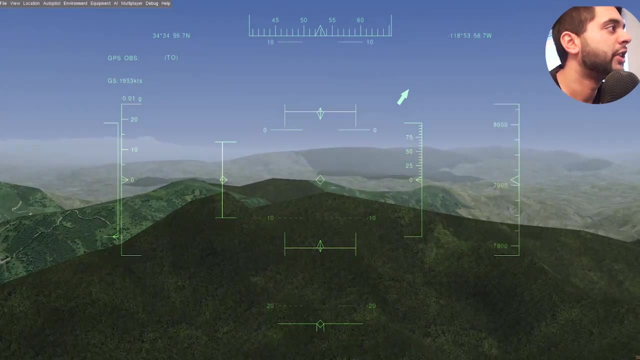 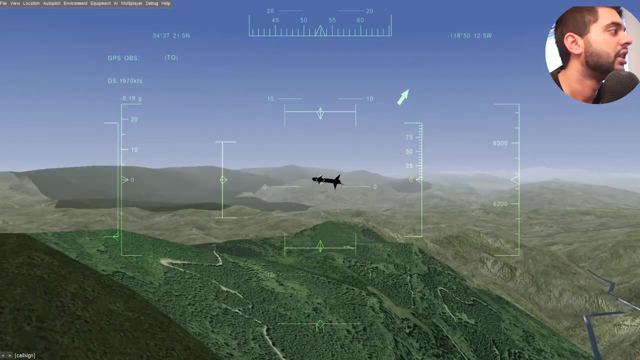 here. so it'll now pitch up and avoid it. so if you take a look, you'll see what it does. so it's almost there at the obstacle. so pitch up now. so it'll pitch up, it avoids the obstacle and then it'll hit the target. so it'll hit the water, as you can see there, and that's.